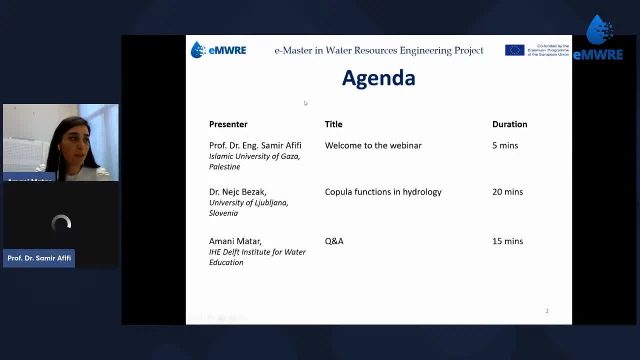 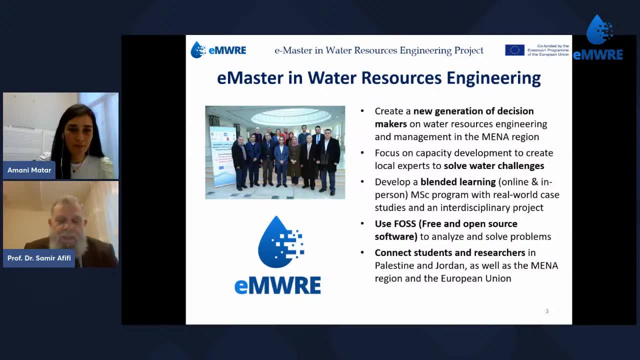 the session. So now I will give the floor for Dr Samir to give you a small introduction on the project And welcome. Thank you, Amani. Thank you, Thank you for this introduction. It is my pleasure to introduce you to the master program. 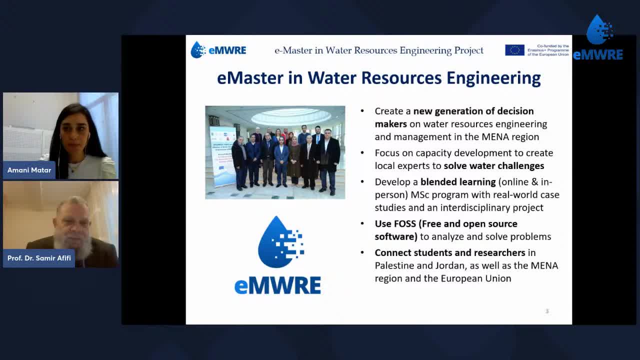 in water resource engineering. The main objectives of this master program was to create a new generation of decision makers. So you know water issue is a very sensitive issue in the area, especially in the Mediterranean area. So building the capacity of the new generation. 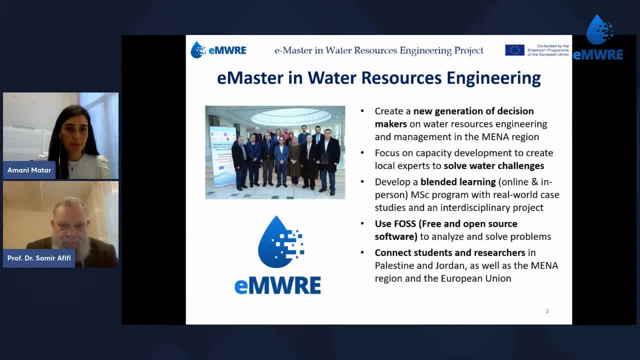 of the decision maker of this area is very, very important And, at the same time, we hope that the expertise will participate actively in solving the water challenge through the many activities which will be introduced in this master program. In addition, the program will be introduced in a blended learning approach. It means that all courses which will be presented 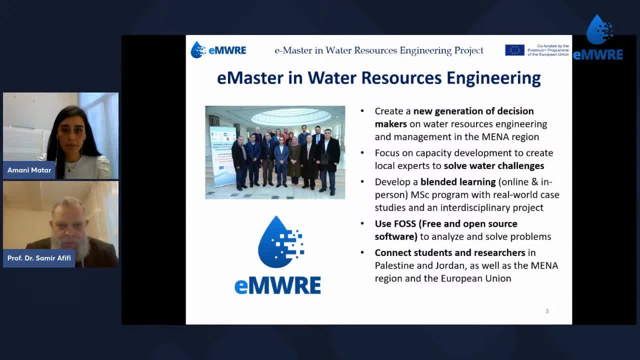 in this master program will be available online. The school will be using free and open‑source software which will be used to analyze and solve a problem. It is very important. Connected students and research in the regions and in the EU countries. It is very important, So the program will give a good opportunity for. 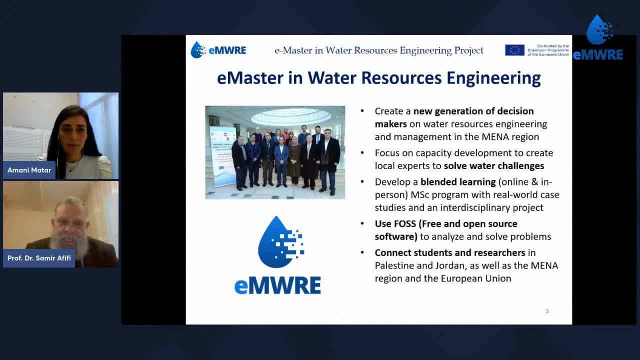 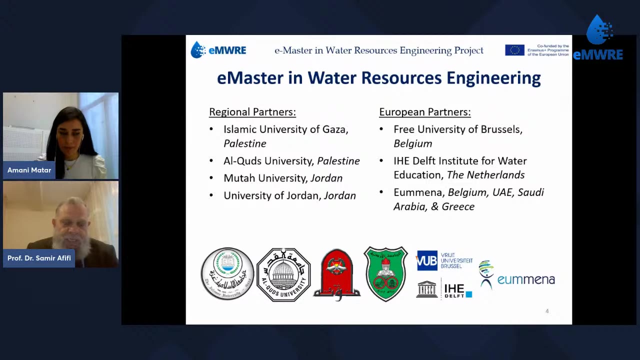 the participant to have and to make use of the regional and international experience in these areas. Many of experts from Europe and from Jordan will participate to introduce some of these courses. Second slide, please. So the E-Master Program in Water Resource Engineering have and hosted a good expertise in different countries. 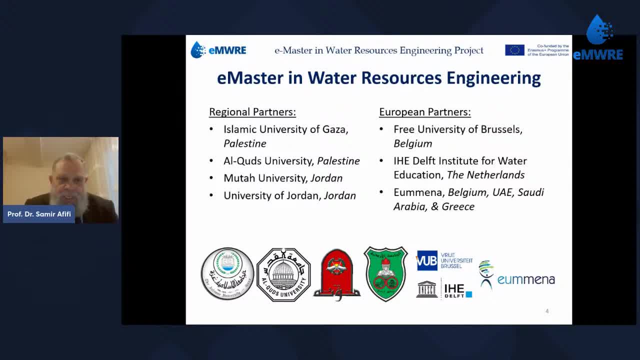 So, in the region of the area, we have two countries with two universities from each one, So we have the Islamic University of Gaza and we have Al-Quds University, both from Palestine, So, and then we have two universities, Mu'tah and University of Jordan, from Jordanian. 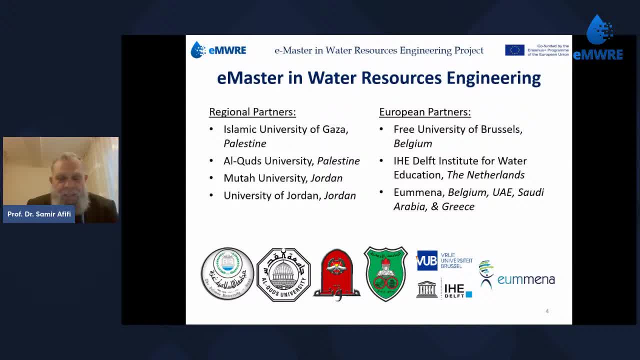 In addition, we have three additional partners from Europe, three University of Brussels in Belgium and IHE Delft Institute for Water from Netherlands, In addition to the very expertise IOMENA Institute from Belgium. As I said, the program is funded. 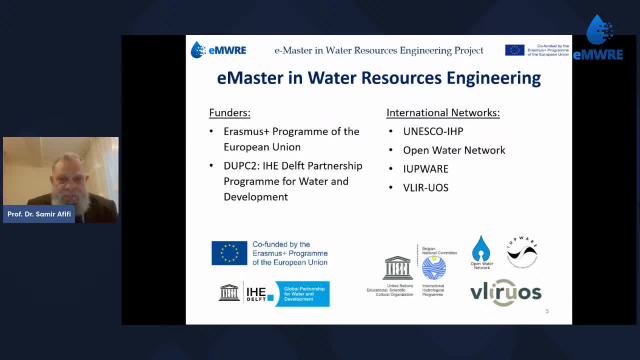 through the Capacity Building Program of the Erasmus mainly, and the Erasmus finance the main activities there. In addition, there is an additional fund from IHE Delft Partnership DUBC2, in addition to the other international networks. 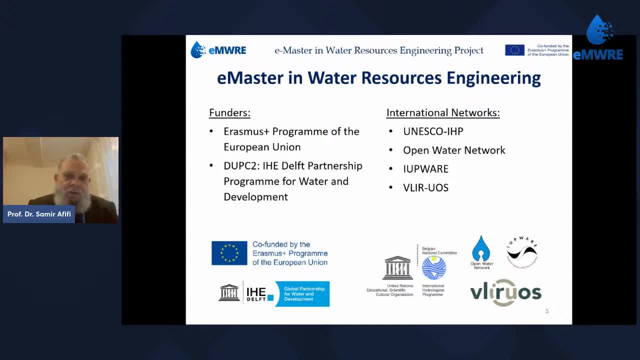 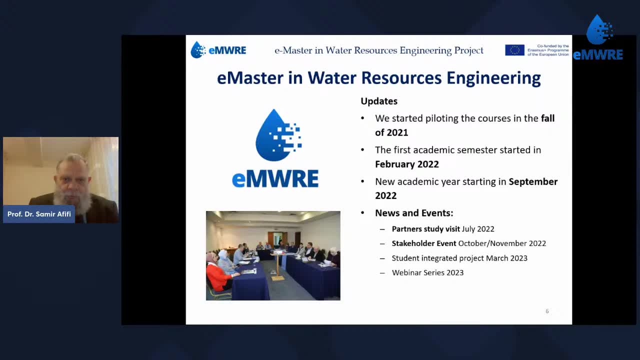 which participated in the financial issue of the project activity. So the Master Program has started with before two years ago and the Master Program is already validated from the Ministry of Higher Education in Palestine And we started last semester to to piloting some courses. 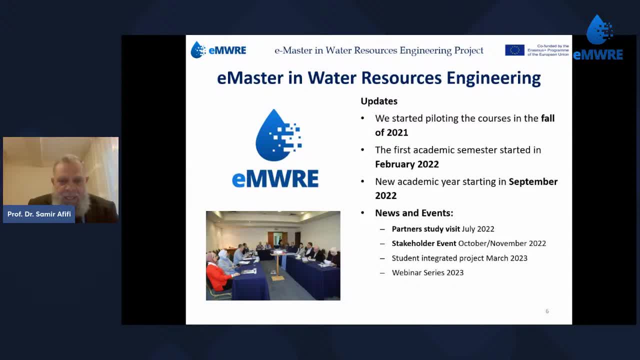 which has already developed in the last two years And in this semester we have already started the program And we hope that in the next semester- September 2022, we will receive another participant in this Master Program. Many new activities is planned for the next phase connected. 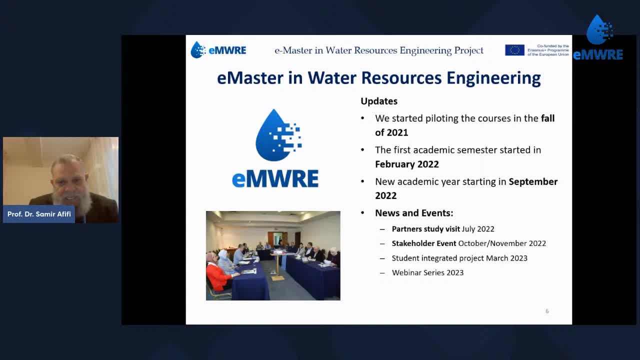 with the study visits, stakeholders events and the third series of the webinar in 2023,. in addition to applying the integrated study project, which will be conducted in Jordan and Palestine, We have highlighted two case studies: one in Jordan and one in Palestine. 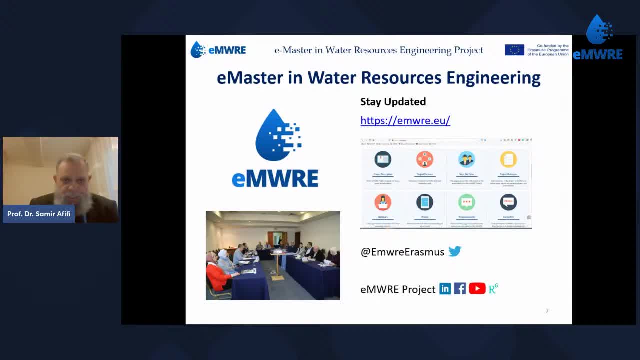 So there is a lot of information presented already in the website and the website of the program. I hope that you can enjoy and see and follow up all these activities within the online and the connected with the link of the program which is presented on the screen. 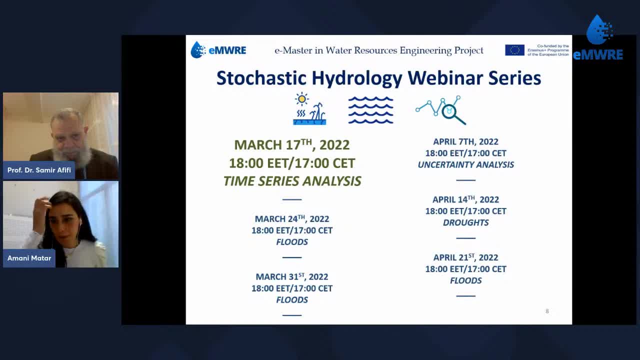 ALINA IVANCHENKOVSKAYA. Thank you, And yeah, so welcome everyone. I see more people are coming in And so, as we mentioned, this is the first webinar series of the Statistic Hydrology. It's mainly six webinars. 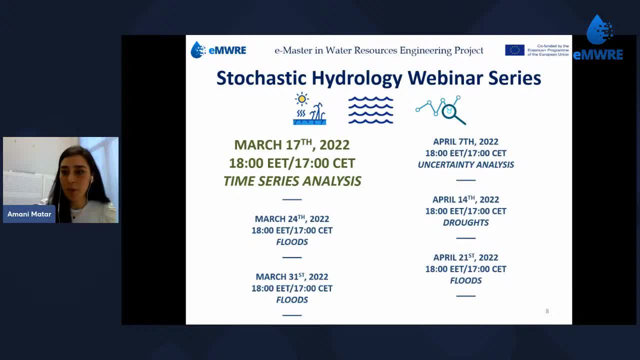 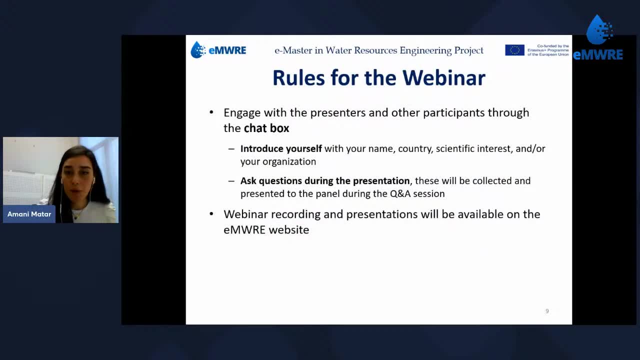 They will be taking place every Thursday from now until six weeks. So we hope you can join all of these webinar series. So we'll just go over the rules of the webinar a little bit. So I see people are already engaging, so please engage. 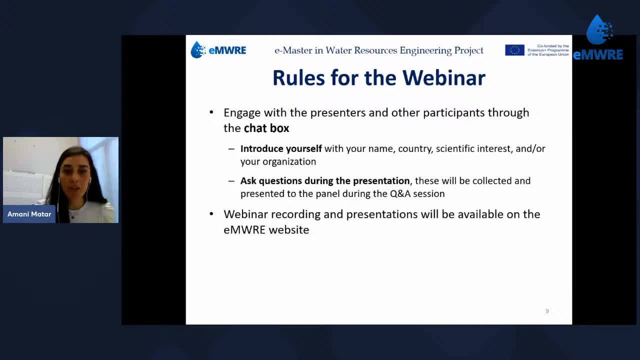 in the chat box. introduce yourself your name, your country, scientific interest and ask your questions in the in the chat box and we will raise them to the presenter and just to find a lot. these webinars will be recorded and they will be available on the project website and social 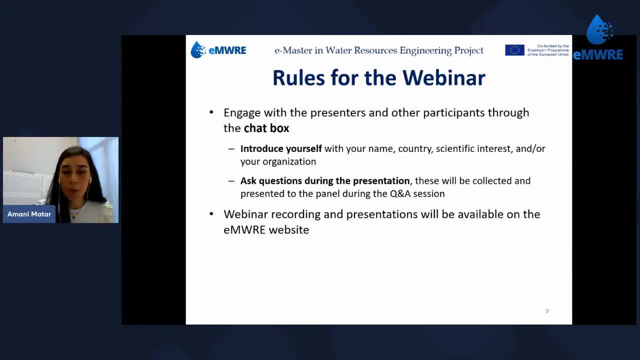 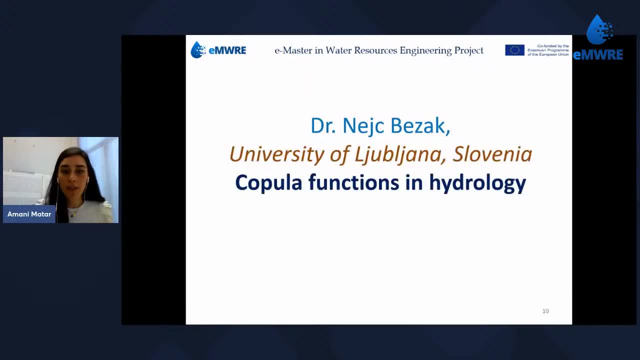 media, as dr samuel mentioned. so please also keep following the project website for more updates and information. so now, so, as we mentioned today, we have a presentation by dr nate from university of lublina in slovenia. so dr nick obtained his master's in civil engineering and graduate diploma. 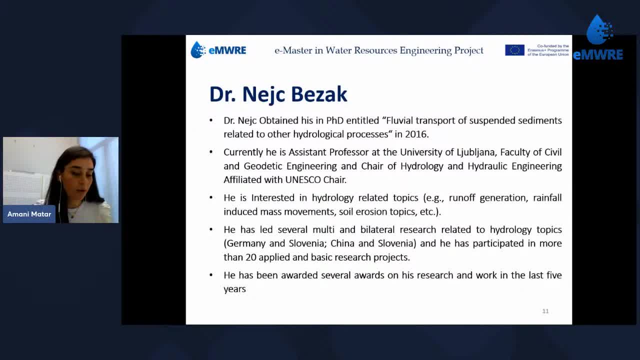 in 2012 and he defended his phd in on fluvial transport of suspended sediments related to other hydrological processes in 2016.. currently, he is an assistant professor at the university of lebanon and the faculty of engineering. he is the chair of the engineering and chair of the. 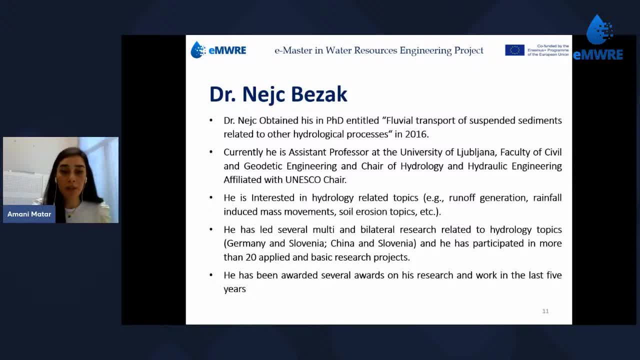 hydrology and hydraulic engineering, and he is affiliated with the unesco chair. he is interested in topics related to hydrology, specifically runoff generation, rain of induced mass movements and soil erosion. he has led several research projects, some of them for the the natural flood retention on private land, and he works on 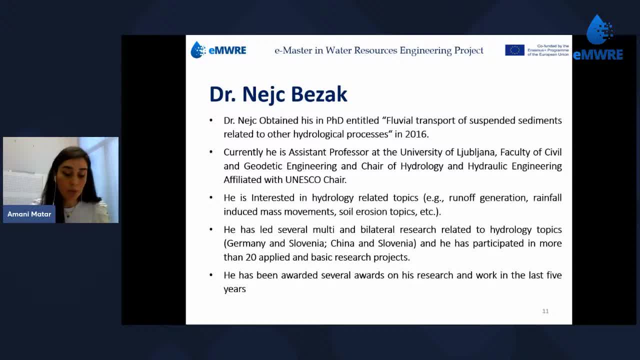 bilateral research projects between germany and slovenia and other projects between china and slovenia as well, and he has cooperated in more than 20 applied and basic research projects, and he has been awarded several awards- several awards for his work, and most recently is the danubian's most young scientist, hour d in 2021, which is issued by the federal 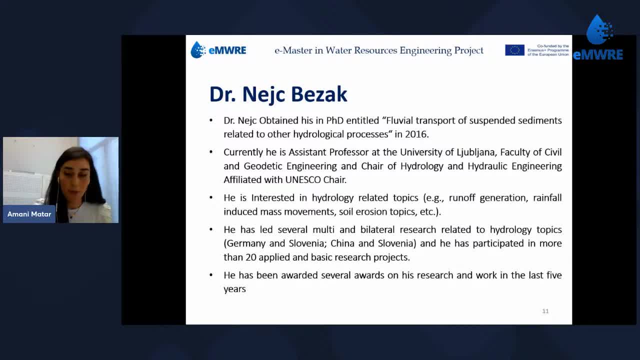 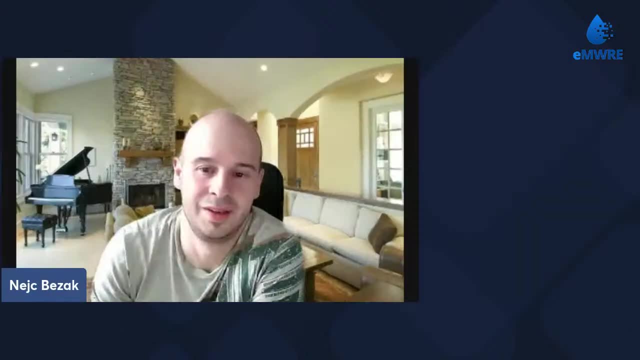 ministry of the republic of austria and other awards as well. so, dr nike, the floor is yours and And everyone. I hope you enjoy the presentation and please engage in that chat, Thank you. Thank you, Amani, for this presentation. Just a second. 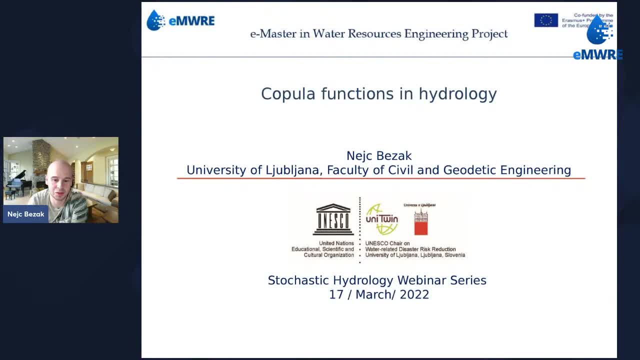 So here should be my slides. So today I will talk about Coppola functions in hydrology, As I was already introduced, so my name is Nate Bezak. I'm coming from the University of Ljubljana, Faculty of Civil and Geodetic Engineering. 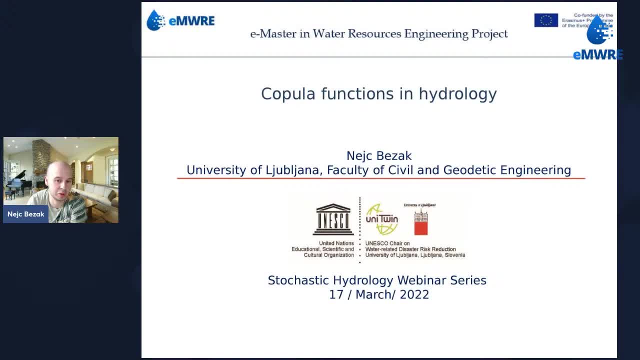 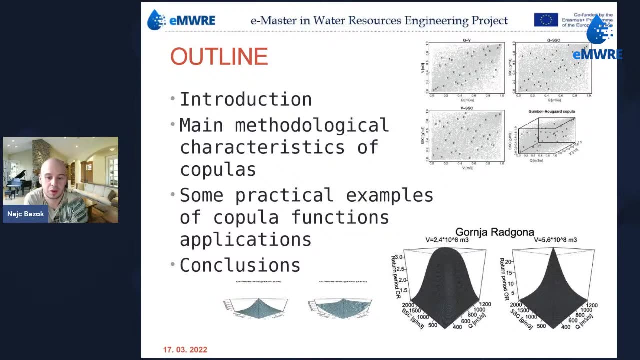 I'm also affiliated with the UNESCO Chair on Water-Related Disaster Risk Reduction. It is also organized in the scope of the same faculty, the same university. So, firstly, a short outline of today's presentation. So I will start with a short introduction. 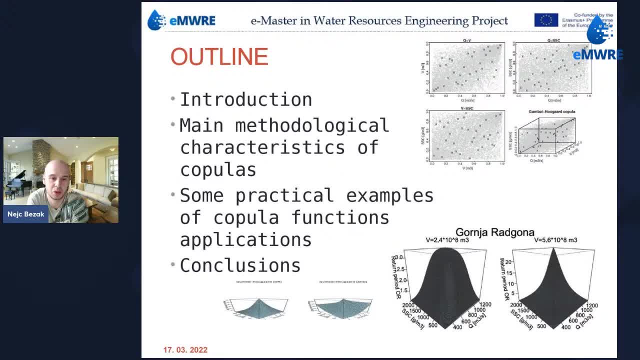 Then I will describe briefly main meteorological characteristics of using Coppola functions. I will talk about the role of Coppola functions in hydrology. So let's get started. I will present two practical applications of how Coppola functions can be applied in the broader field of hydrology. 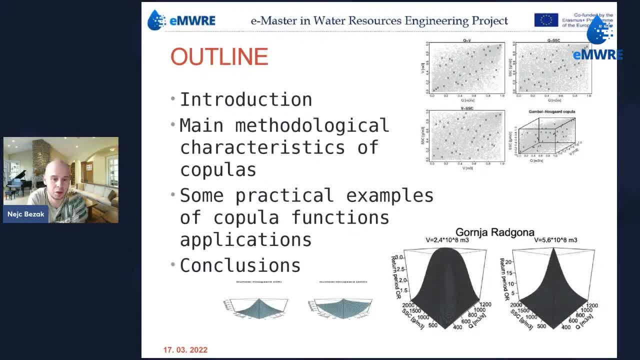 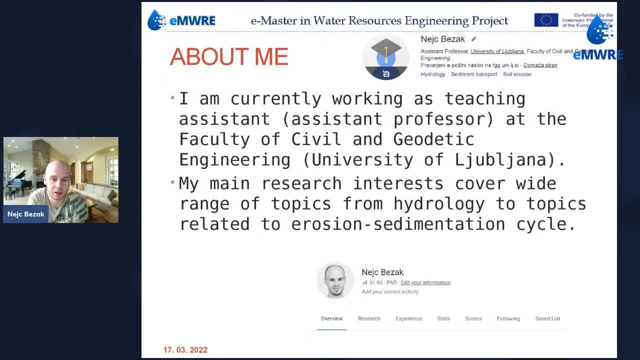 And I will conclude this presentation with a few thoughts, final ones. So shortly about me. So, as it was said, my research, basically activities, cover a wide variety of topics. hydrologic, from hydrology to erosion, sedimentation cycle and so on. 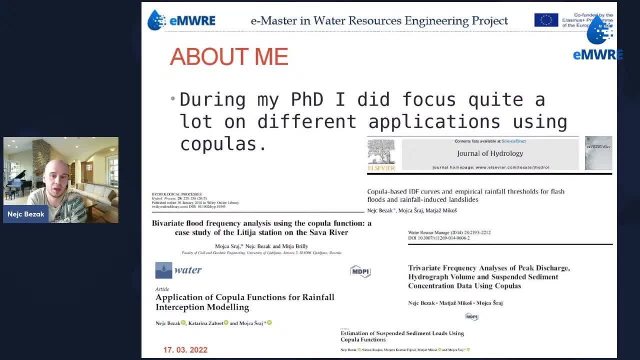 So during my PhD I did focus quite a lot on different applications using Coppola functions, So I used them for bivariate frequency analysis. I tried to combine sediment data with flood data and model it with Coppolas. I did use Coppola functions for rainfall interception estimations and also tried to try to combine Coppola functions with empirical rainfall thresholds. 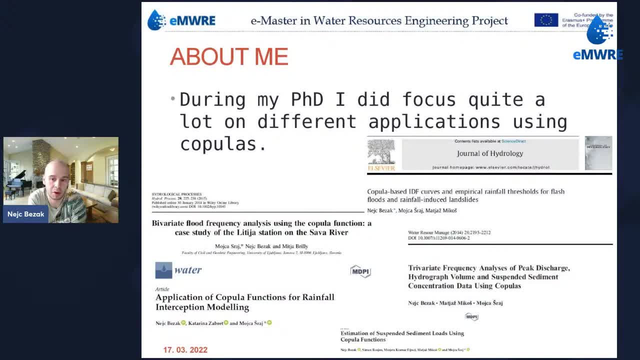 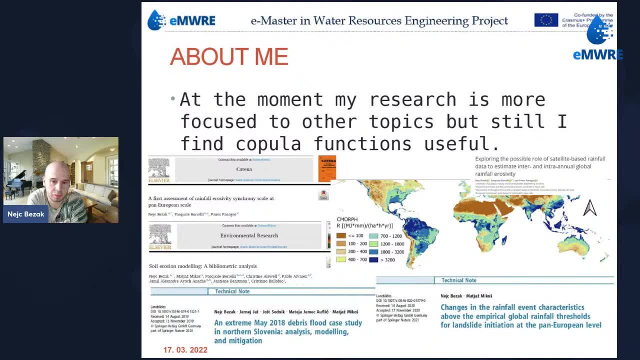 So these are the thresholds. These are the thresholds that can be used for, let's say, empirical prediction of shallow landslides and debris flows. At the moment, my research is more focused on some other topics, especially on this erosion sedimentation cycle. 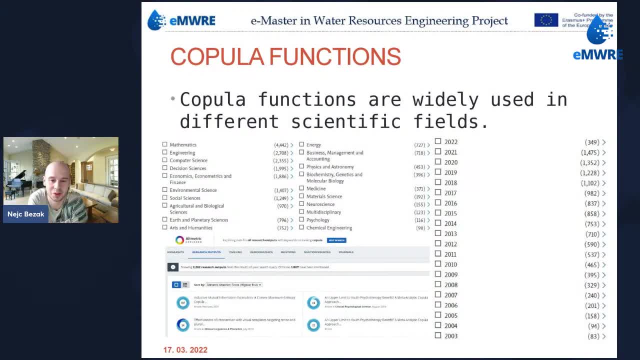 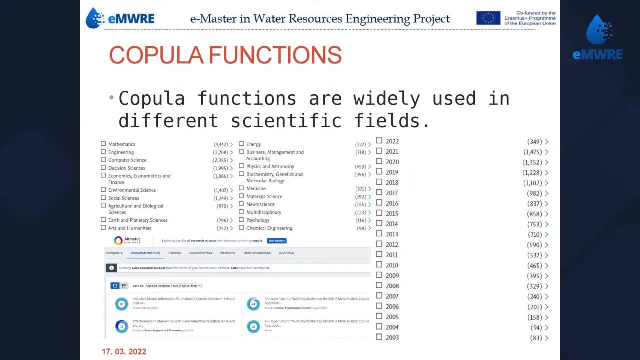 So some of the recent papers can be seen on the screen. OK, so enough about me, Let's go to Coppola functions. So these are basically print screens from Scopus. So as you can see here On the left side. So the search, the search keyword, was basically Coppola functions. 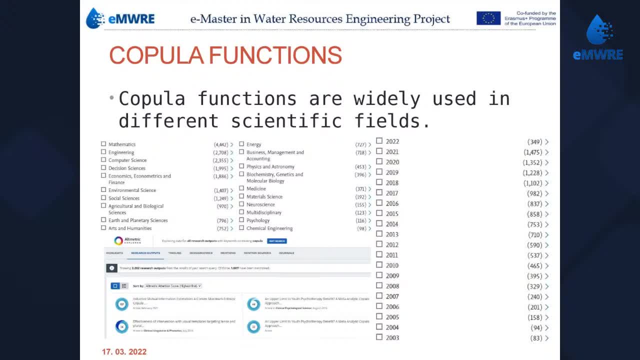 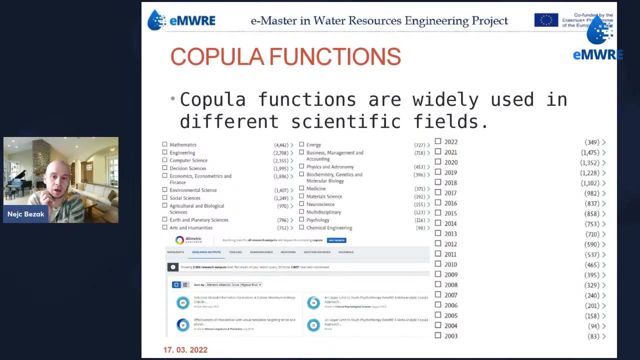 So, as you can see, like the largest number of entries in the Scopus database with respect to the Coppolas is related to the mathematics field. So this means that Coppola functions are actually very live mathematical research area and a lot of research is done in relation to Coppola. 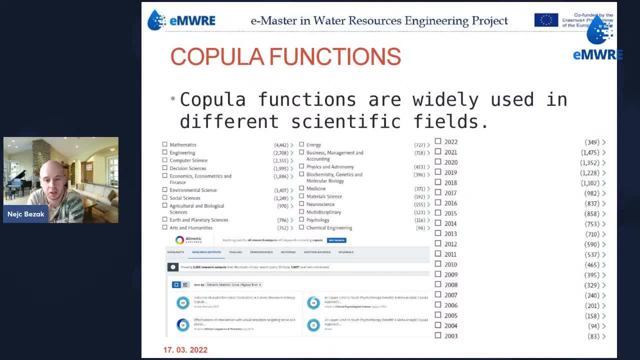 So this means that you Coppola Functions are being developed, new tests are being tested, new approaches and a lot of stuff is is still under development. So you can see on the right side it's the number of publications or the number of entries in the Scopus database is steadily increasing. 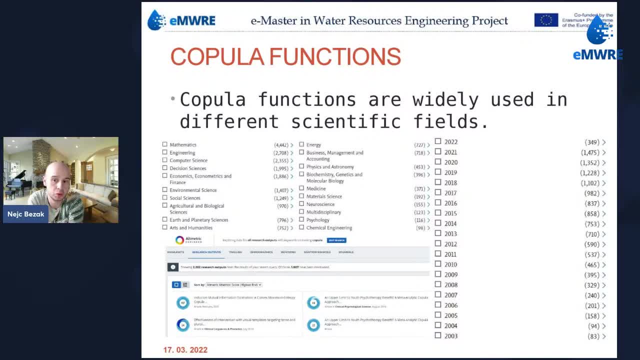 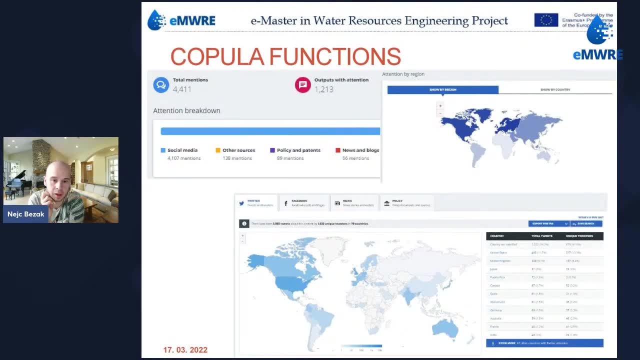 So every year there are more and more publications that do use Coppolas for different things, And another thing that I wanted to show. so this is the. This is again similar search, so using the Coppola function search term, but this time it's using the altmetrics explorer. 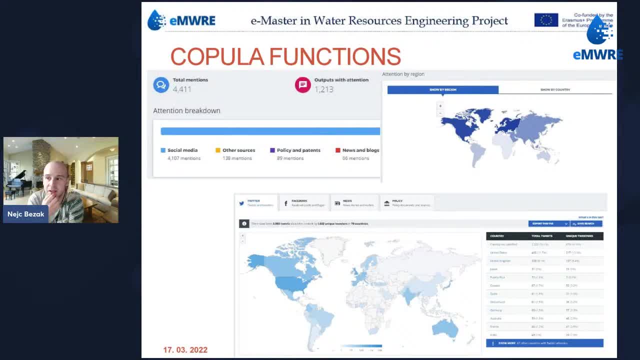 So the altmetrics is basically, let's say, a search engine that relates research outputs with social media tracking, with policy patterns, news blocks and everything. So you can see that mostly Coppola functions have quite a lot of attention. So, especially in relation 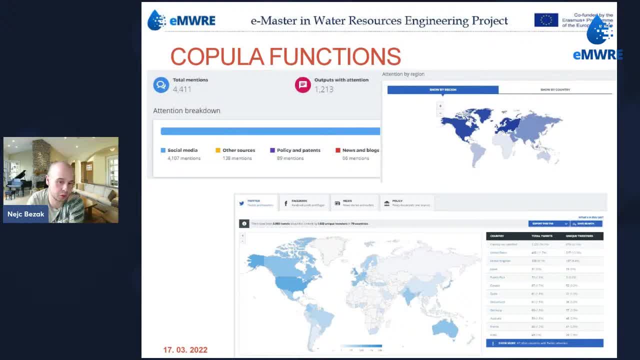 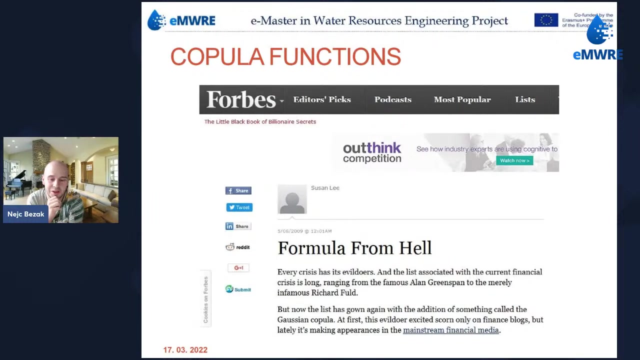 To Twitter in the North America, Europe, Australia, South America and also India and also some other Asian countries as well. So the topic is basically very international And, as I said, it's still developing, but it's. it was not that positive in the past. 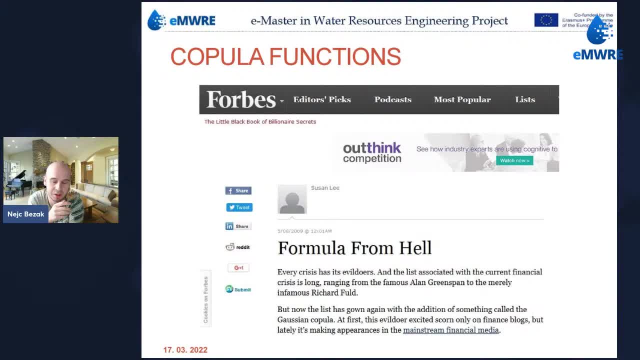 So I think that this paper, if you're interested in it, Can still be found on the web. So basically, Coppola function or, more specifically, Gaussian Coppola, So the normal Coppola was basically- at least these were speculations- of the modeling. using the Gaussian Coppola was one of the reasons for a big financial crisis. 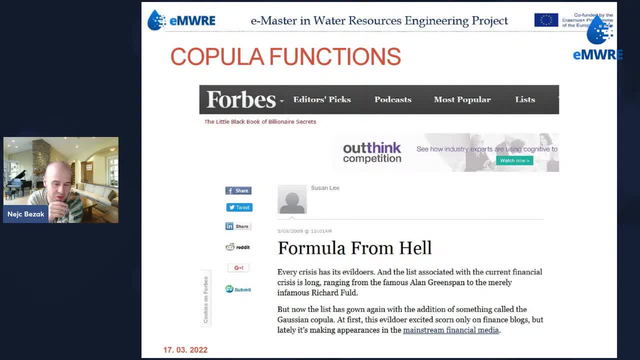 So the global one that occurred in the years 2007, 2008.. So, as you are, if you are interested in it, you can find it on the Web page, So you can Google it And you can read it and find more information. 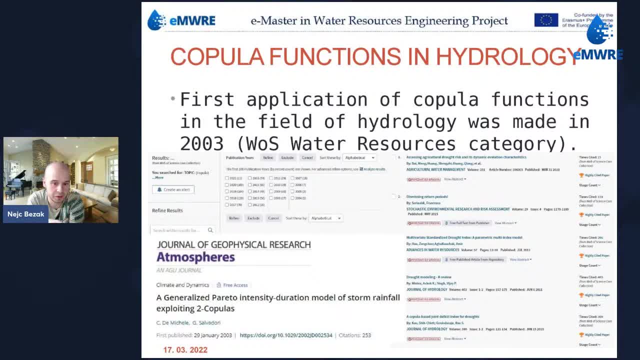 So coming more specifically to hydrology field. So the first application of Coppola's in the field of hydrology was was done in year 2003 by Carla de Michele and Juan Fastos Salvadori In this paper where they modeled the intensity, when they constructed the intensity duration model of storm rainfall using two dimensional Coppola. 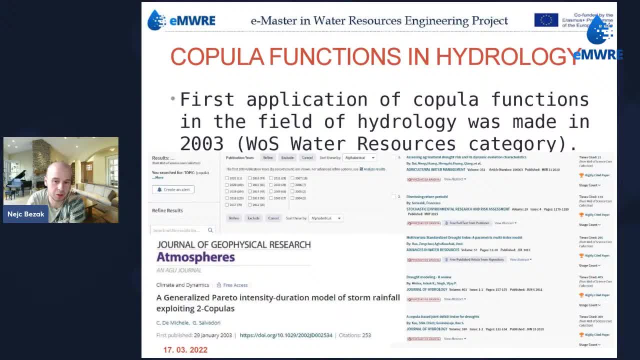 You can see also that also in the field of the water resources, so in the field of hydrology, the number of locations that do use Coppola sees like steadily increasing, And you can see on the right side of the screen that a lot of these publications are also like labeled as highly cited papers by that of science. 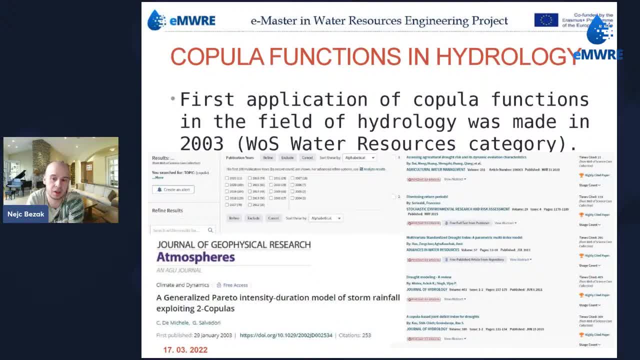 So this means that, like this kind of papers are attracting a lot of attention by the scientific community, especially in the field of drought assessment. So, as you can see here, five or four of these four or five papers that are labeled as highly cited papers, 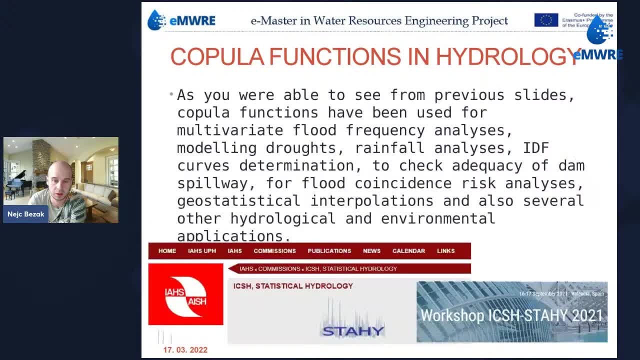 are using copulas for drought assessments. But not only can copula functions be used for drought assessments, they can be used, as I said, for bivariate, multivariate flood frequency analysis, rainfall analysis, intensity duration, frequency curves. 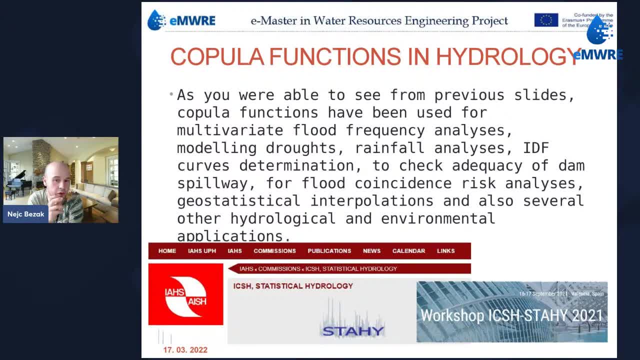 determination to check the adequacy of dam spillways for flood, coincidence risk analysis, geostatistical interpolations and so on. So, if you are interested, so there actually exists an organization that is called STAHI and is basically organized under the umbrella of IHES. 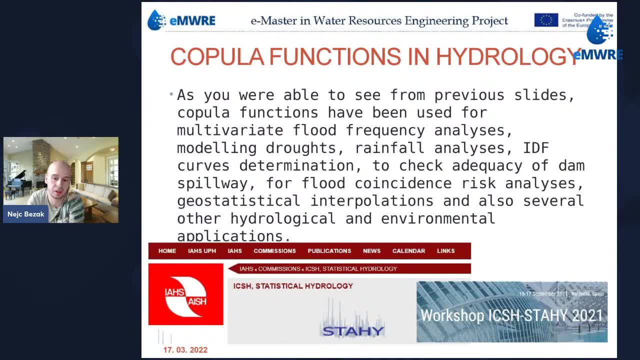 And STAHI does organize, like periodically conferences, and within these conferences or separately, there are also organizing workshops. So the last workshop was actually organized last year. It was done virtually in. it should be done like in person, in Valencia, in Spain. 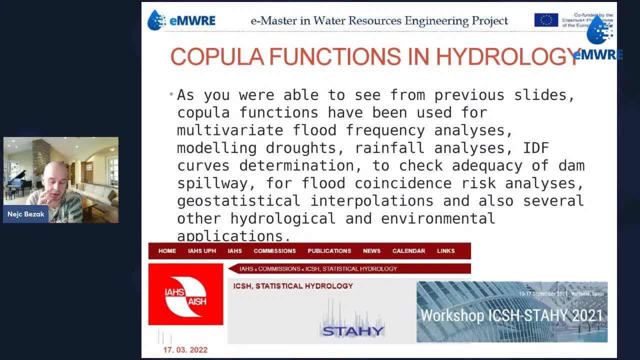 But during these workshops a lot of attention is given to copula functions And in the past there were actually specific workshops dedicated. so one week workshops dedicated to copula functions, So how to use the theoretical background and so on. So you can check the webpage. 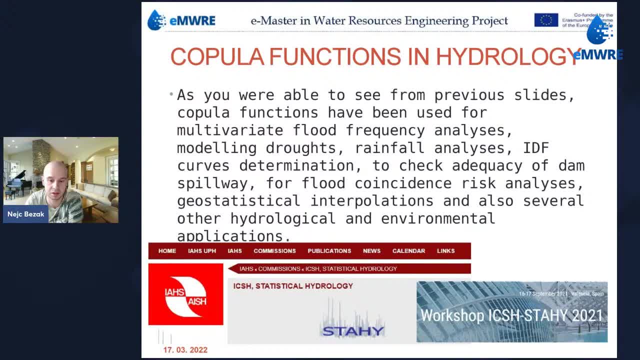 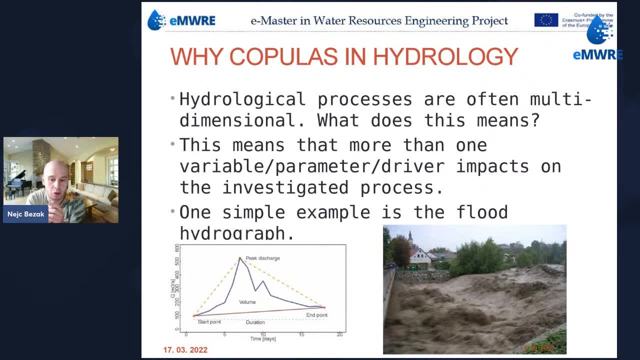 and perhaps there will be further events in future. if you're interested to get more information about it, Okay, So why should one use copula functions in hydrology? So the reason is because the hydrological processes are often impacted by different let's say: 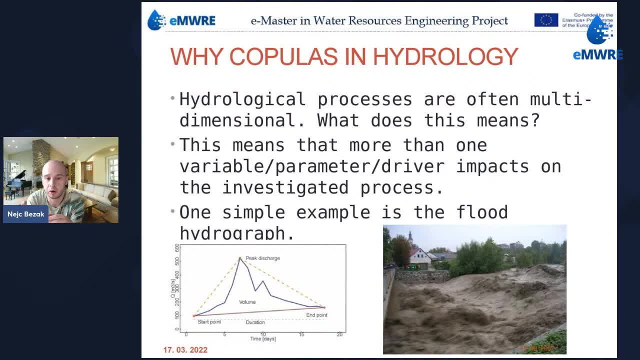 outside processes and or different drivers, or specific characteristic is basically can be characterized by like multiple variables and so on. So one simple example is the flood hydrograph. So if you're dealing with hydrology, you all know it. So usually one simple example is the flood hydrograph. 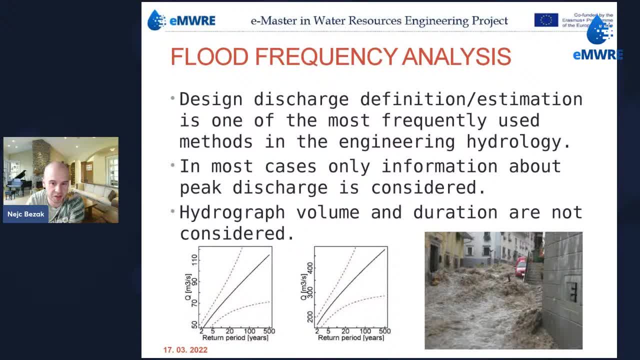 So if you're dealing with hydrology, you all know it. So usually one simple example is the flood hydrograph. So you can see here what is used in the like flood frequency analysis, Since flood frequency analysis and determination of the design discharge is one of the steps. 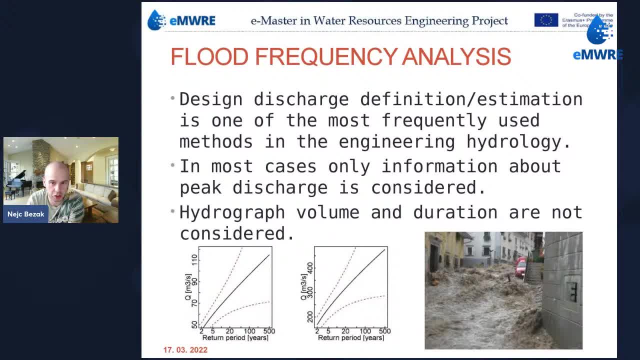 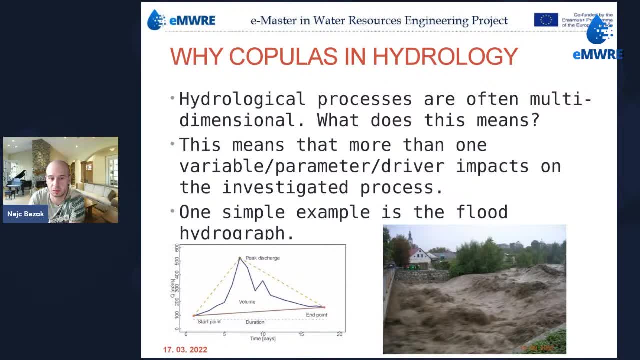 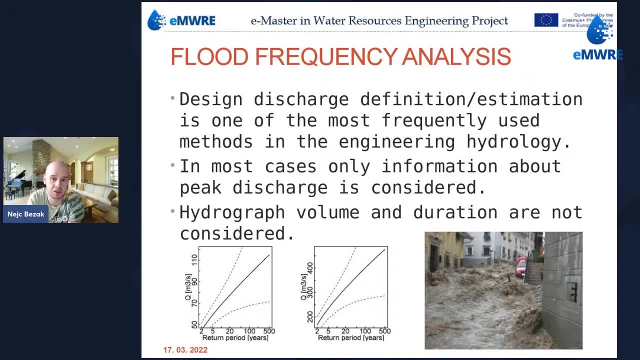 that is most frequently used in the engineering hydrology. So what we usually do in flood frequency analysis we only select, like the peak discharge values, so the maximum one from the specific years, And we do the univariate flood frequency analysis. So this means that we only consider the peak discharge values. 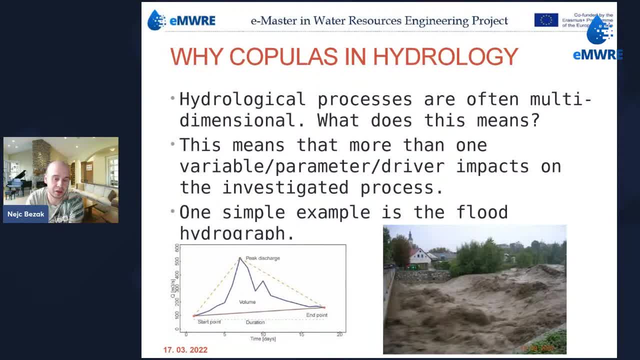 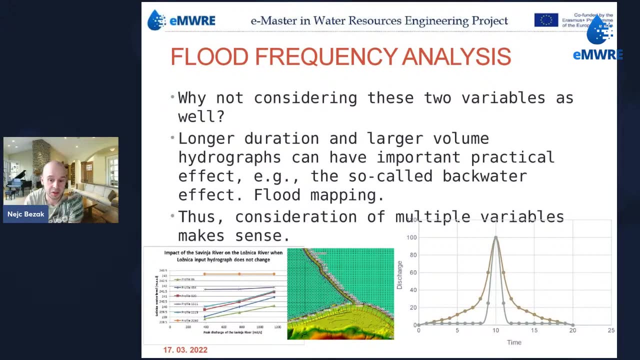 discharges and not also the other characteristics of the flood hydrographs. So this means that flood volume and the flood duration, as two important characteristics, are not considered in this process. So why is this important? This is important because, as you might imagine, so the hydrograph volume and the 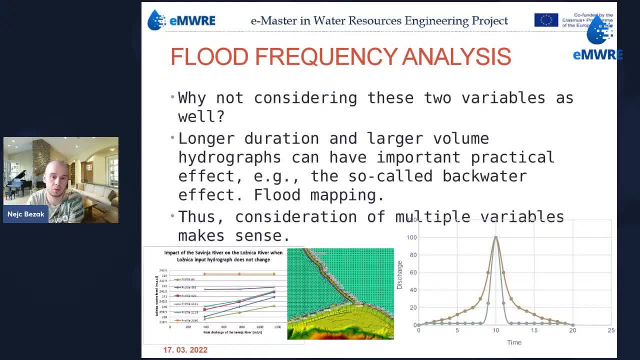 duration does have effect on a lot of things. So flood mapping it does. basically, it is related to the, not only to the peak discharge, but also to the, to the, to the volume and duration, For example, the backwater effect and everything and all the steps, for example, 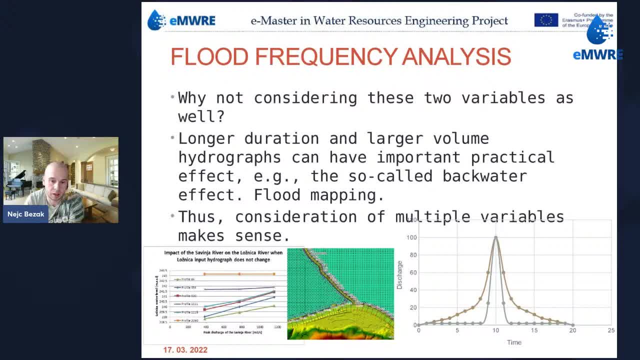 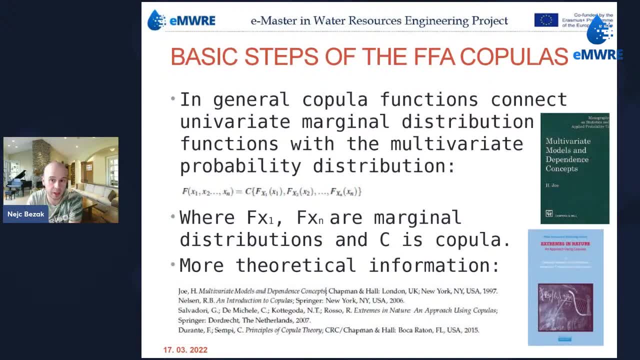 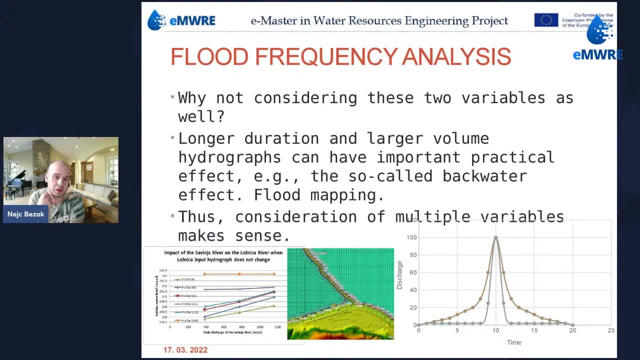 that are needed in the flood risk mapping are somehow related to the, also to the flood duration and flood hydrograph. So why not using also this, These two variables, in the process of flood frequency analysis? so Coppola functions can help here, So bivariate or multivariate flood frequency analysis can be done in order to 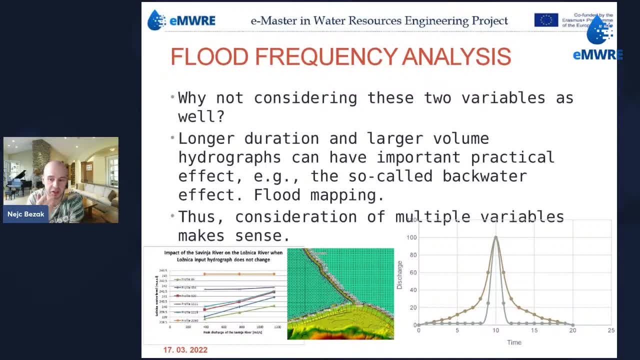 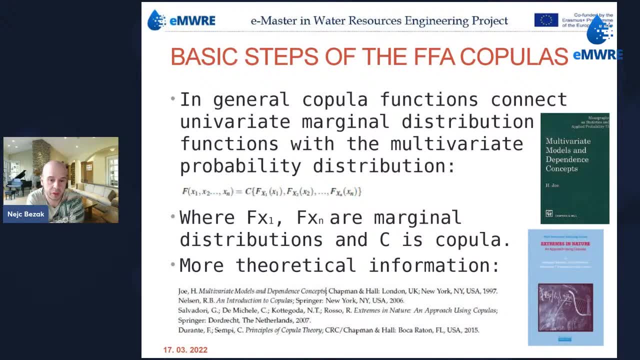 to basically also use this information in the design process. OK, so a lot of theoretical information can be found in the classical textbooks. since this is quite short presentation that I'm delivering Here today, I will not go into very details of it. 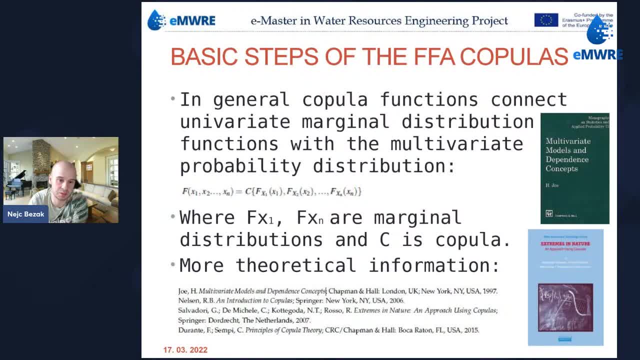 So if you're interested, I would suggest these textbooks that are mentioned here, So especially this one that is entitled Extremes in Nature. an approach using Coppola is very useful, But in general. so the Coppola functions, the Coppola function, do connect the 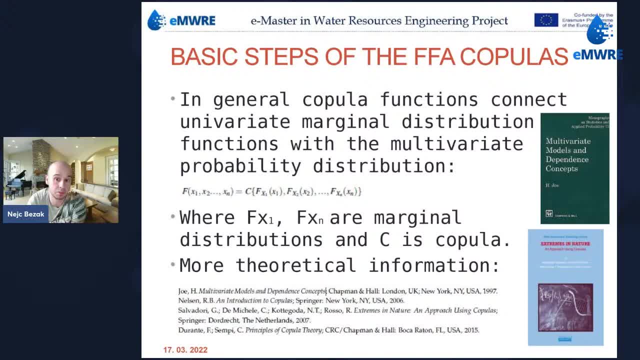 univariate marginal distribution functions with the multivariate probability distribution. So this is basically the equation, This connecting where one uses Coppola to in combination with, with univariate marginal distributions in order to to somehow combine this multivariate or information from different For different, let's say for different aspects. so 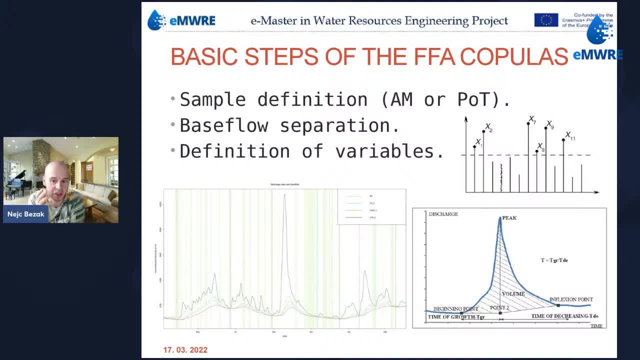 I will focus on one example, so basic steps, of the bivariate or three variate flood frequency analysis, analysis using copula functions. i will go like briefly to the basic steps so that you will perhaps better imagine how copula functions can be applied in order to conduct the multivariate. 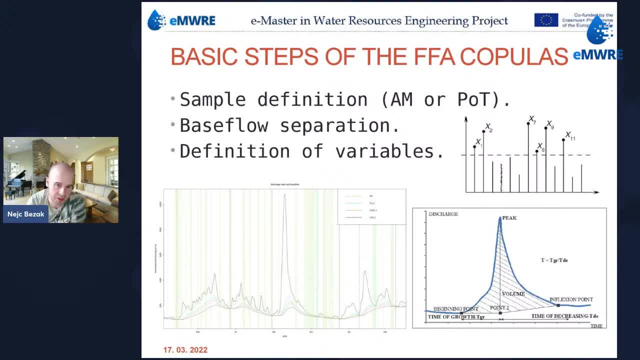 flood frequency analysis. so the first step is, similarly as in case of the univariate analysis, sample selection. so here one can use the annual maximum method, so selecting the maximum peak per year, or the pixel over threshold method, where one selects more events per year. the second step 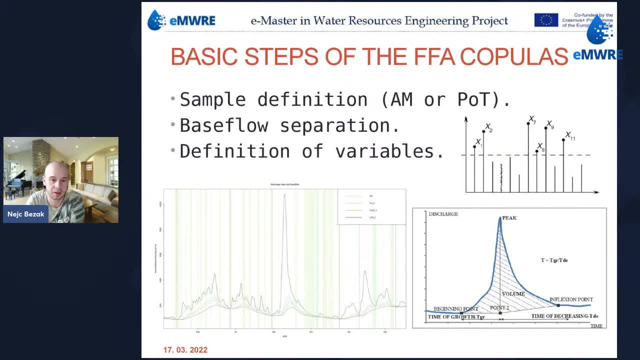 is base of separation. so here we should like separate the surface flow from the base flow in order to consider only this surface flow in the process of the multivariate analysis. so here again, different methods, different different digital filters or simple methods like this one using the three-point method. 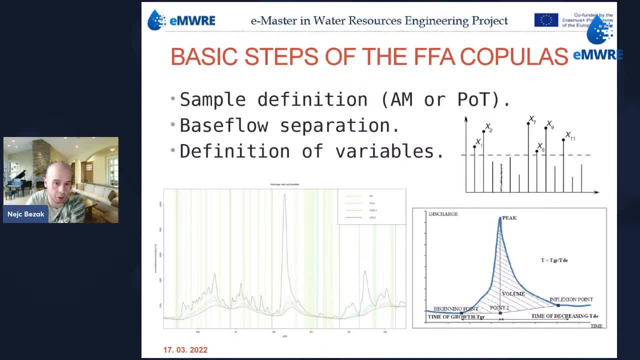 that can be used to to define the, the hydrograph body. so after we have, like, separated the base flow or estimated the base flow, we can determine or calculate also the hydrograph volume, which is basically the area under the hydrograph, and we can also calculate the hydrograph duration, which is like the duration, the time duration. 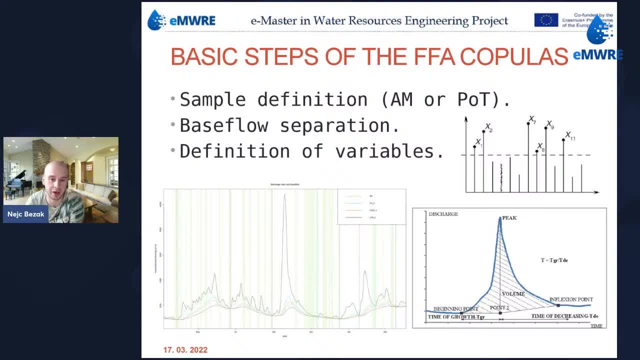 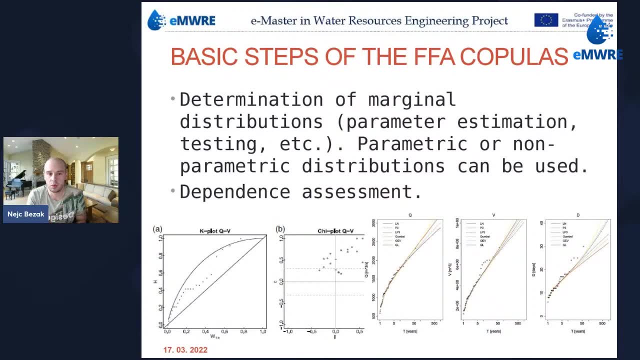 between starting point and the ending point of the hydrograph or the ending point of the surface flow. perhaps better to say, then one needs to estimate the marginal distribution. so marginal marginal distributions are actually similar the same distribution functions that are used in the univariate analysis. so these are, for example, normal distribution, generalized extreme value. 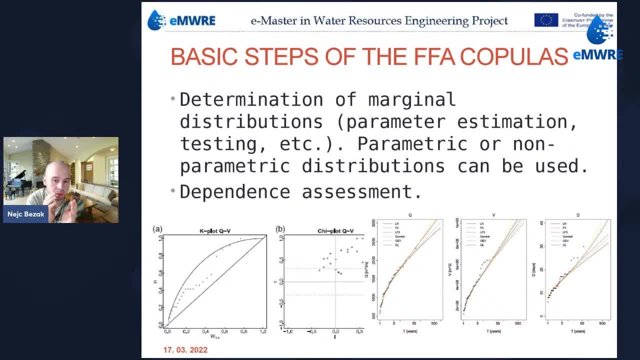 distribution: pearson type 3 distribution. so every variable that we want to use in the process is basically described with one univariate or marginal distribution function. so in this case you can see examples for the peak discharge, for the hydrograph volume and for the hydrograph duration. so again, parameters. 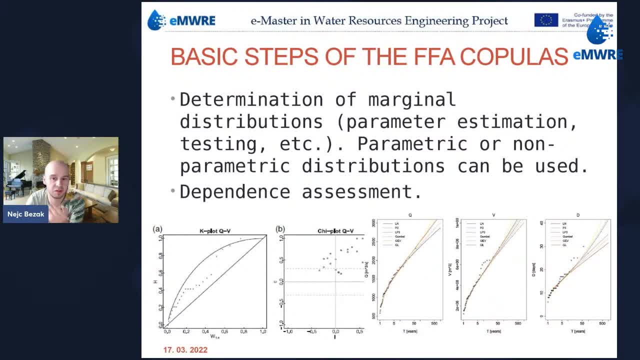 parameters of these distributions need to be estimated. we have different uh methods here: method of moments, method of l moments, maximum server likelihood method and so on. we need to, of course, step, we need to of course test if the selected distribution does fit to data well, so, using statistical tests or goodness of fit criteria, we can do that. 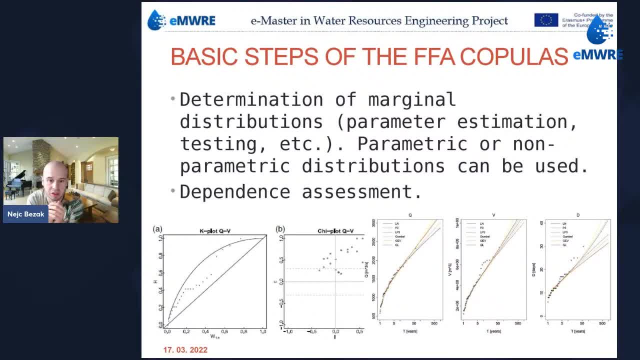 If the parameter distributions, like normal distribution, are not fitting to the data, well, we can also use the non-parametric distributions that are the alternative. Then the next step is the dependence assessment. So we should assess the dependence between the pairs of variables, so between the peak discharge, hydrogen volume. Here there are different graphical representations. 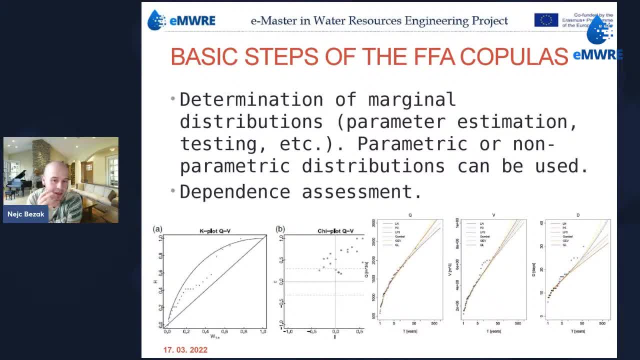 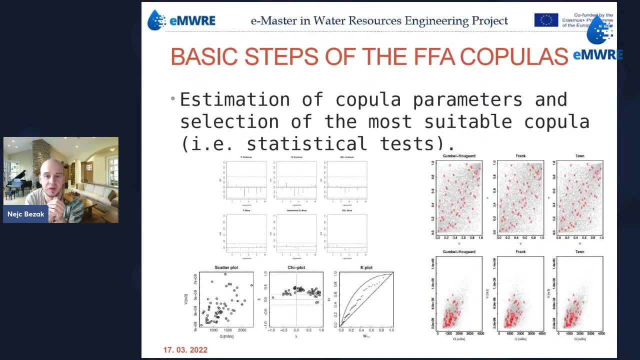 tests that can be used to do that. As I said, like the, the field of Coppola functions is actually very live and a lot of mathematical concepts are still under development. Next step of this multivariate flat frequency analysis is basically selection or testing of different Coppola functions. 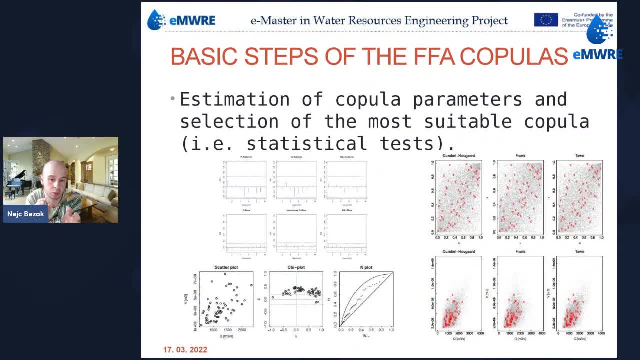 Here again, we have specific tests, how we can check if the specific Coppola does fit to the data. well, We have some graphical representations, like the ones shown here in the on the right part of the screen. so where we have, like the gray points- A lot of gray points- are basically the simulated 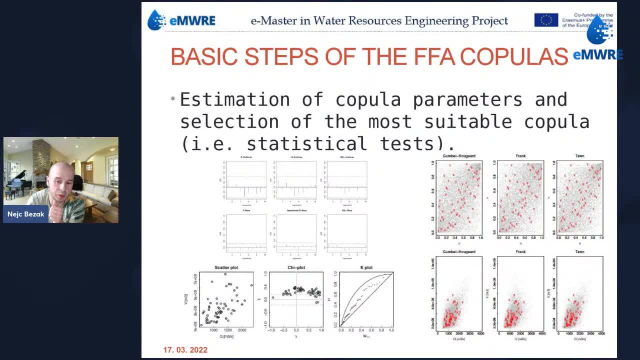 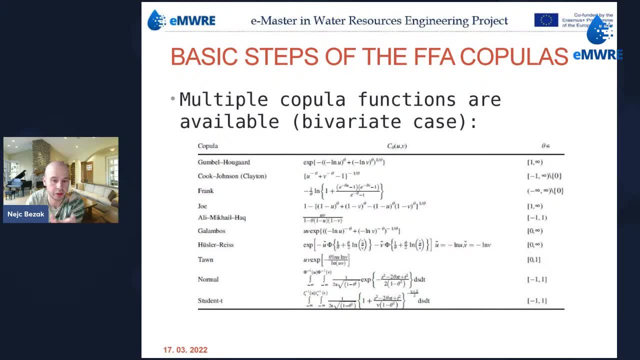 values using the fitted Coppola function, while the red ones are basically the measured data. So there are actually a lot of Coppolas that are used in the field of hydrology, more specifically, for the multivariate flat frequency analysis, like the ones that are shown on the screen, are perhaps one of the most frequently used. 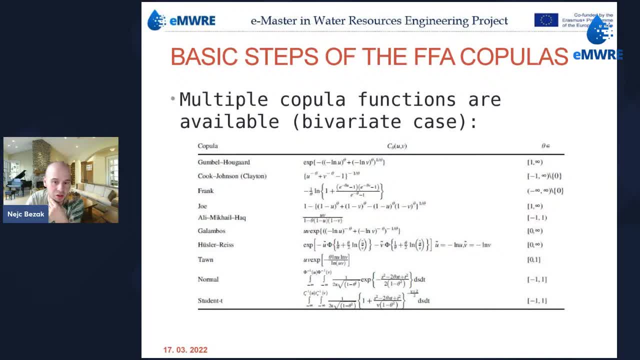 So, as you can see, each of these Coppola functions has its own characteristics, its own range of the parameter, and you should be aware that these are only the functions that are basically characteristic for the multivariate flat frequency analysis. So we can see that these are the equations that are valid for the b-variate case. 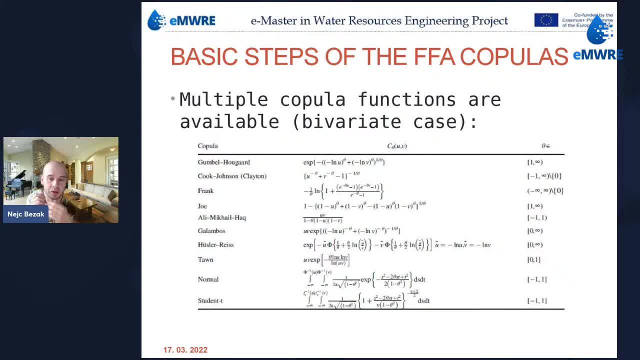 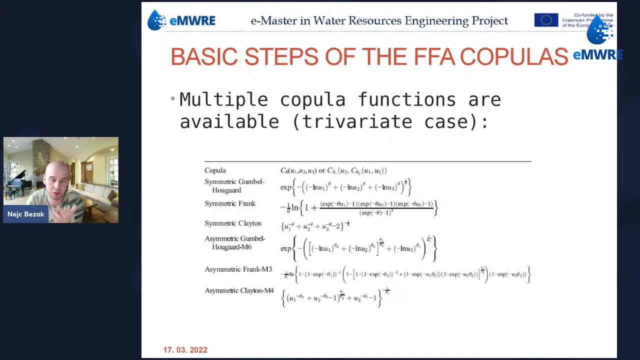 So this means that if we want to consider only two variables, two parameters at the same time, so, for example, peak discharge and hydrograph volume at the same time, While if we go from the b-variate to the three-variate case, so this would mean that 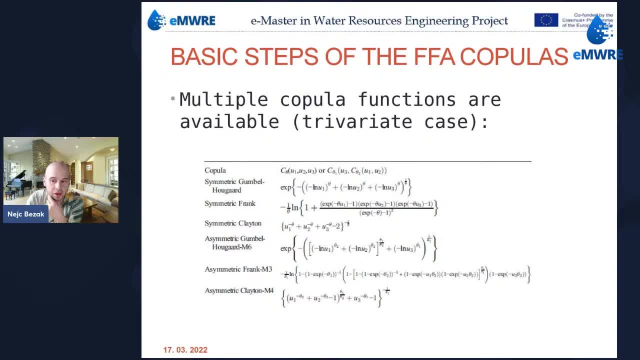 also connecting the hydrograph duration in this investigation, then the equations do become a bit more complicated. So these are also some examples. As you can see, then you can have either symmetric version of, for example, Gumball Coppola or the asymmetric version of the Gumball Coppola, While, as I said, like there are different specifics of 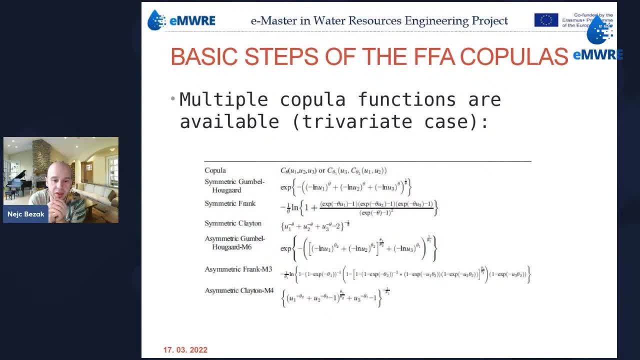 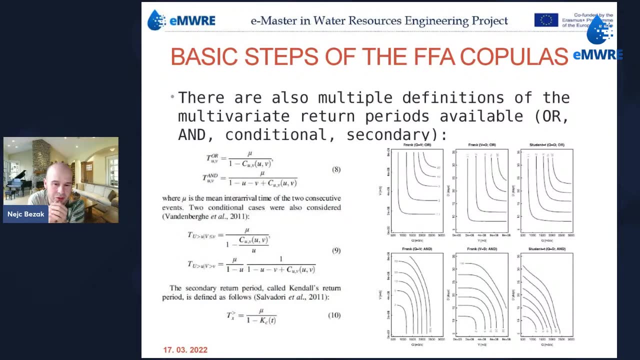 each specific Coppola function. If you are interested in it, you are able to find a lot of information in the previously mentioned textbooks. Okay, so, basically then, the final step is the selection of the return periods. This is perhaps the most tricky step since the notation of the return period to the, for example. 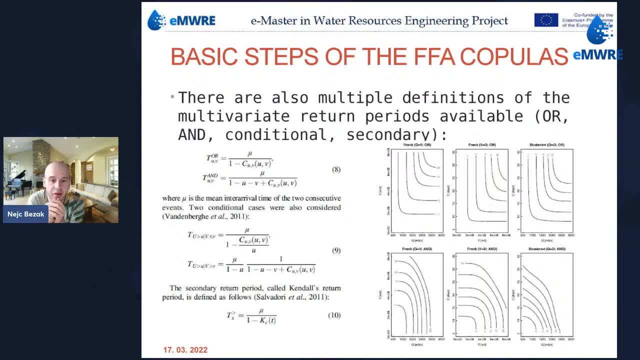 the b-variate one or any other multivariate one is not similar as the notation of the return period used in the univariate case, So I will mention only two cases that are perhaps most easily understood. So these are so-called or and so-called end return periods. 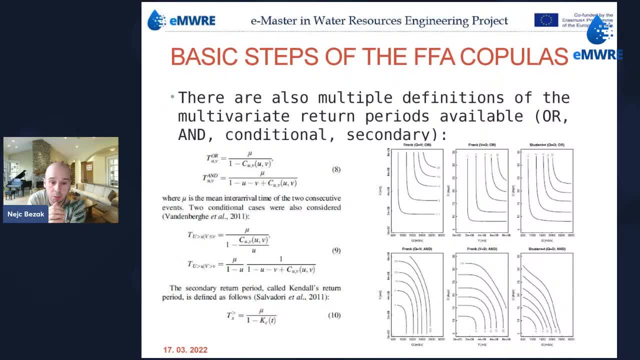 So while there are other definitions available, so as example, different conditional return period, secondary return periods and so on. So or and end return periods are perhaps the most easy to understand. So the or basically means that one or the other or both variables should occur to reach basically the specific return period, While the end does indicate the 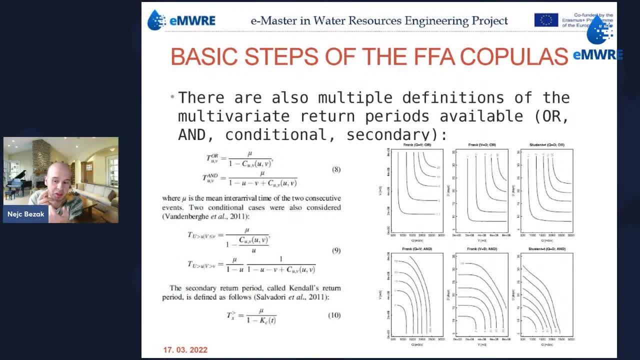 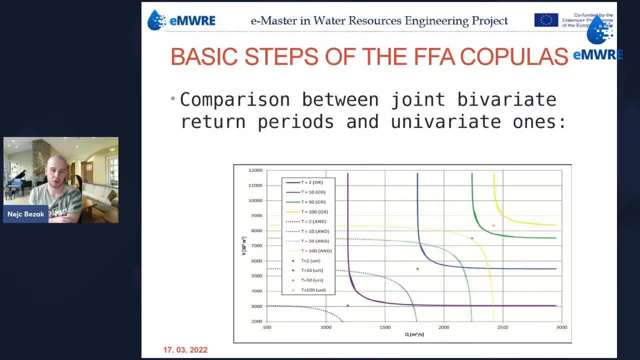 case where both variables- so also, for example, peak discharge and hydrograph volume, should occur at the same time. So I will show an example of a comparison between the univariate case, so the univariate return period. So these are basically the points that are shown on the on the graph. 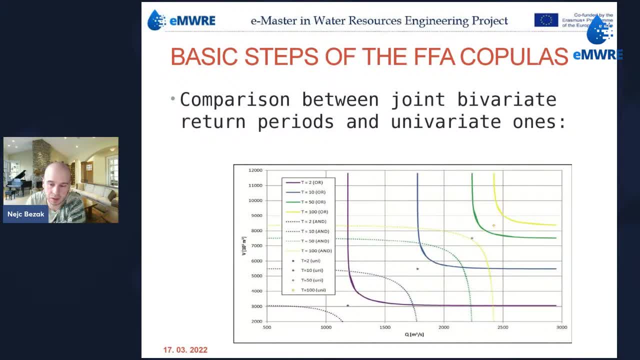 So the colors are perhaps not that well shown. So, for example, like higher one that is shown in this plot is the 100 years one. So this is the yellow point. So in the univariate case we have like one point that does describe the 100 years return period. 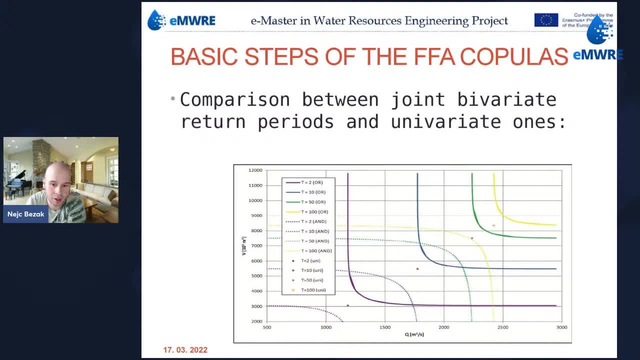 for the peak discharge, which is on x-episodes, and 100 years for the flood volume, which is on the y- axis, While in the bivariate case we can have either the entry term period, so this is the dotted yellow line, and we can have either the all return period, which is full yellow line, So you can see that the 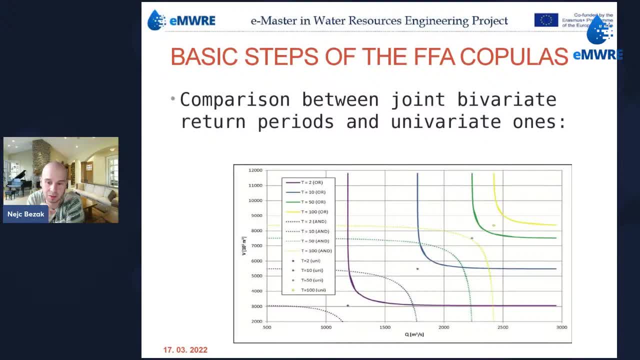 univariate return period always lies in between the air and the on end case. So this is like. I will say a few words also later on. this is perhaps the most tricky point of you of doing like multivariate frequency analysis, since these things need to be explained to the decision makers, to the stakeholders, to the people. 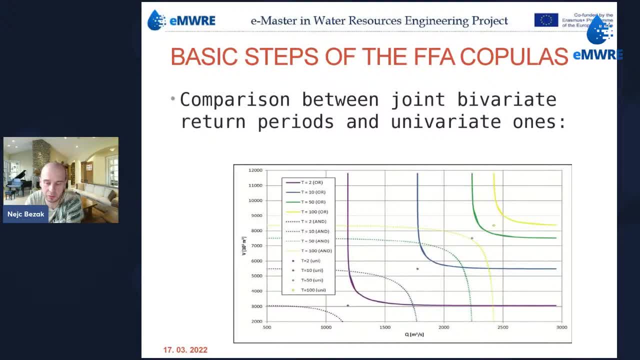 involved and perhaps and sometimes it's hard for them to understand what these bivariate return periods means. Especially, as you can see here, for the bivariate case, you can have different combination on the peak discharge and the height of the volume that are associated with the same. 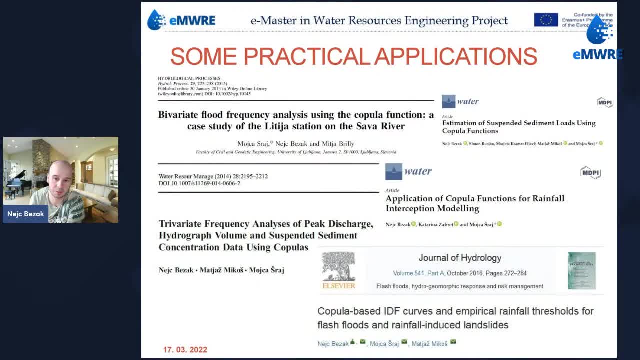 value of the return period. So this is perhaps sometimes a bit tricky. So, as I said, some practical application. so this is a little bit of a test. So this is the bivariate return period. so this is a a promotion of my previous papers. if you're interested in it, you can search. 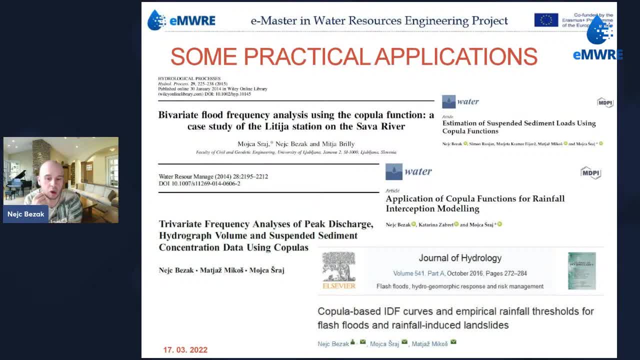 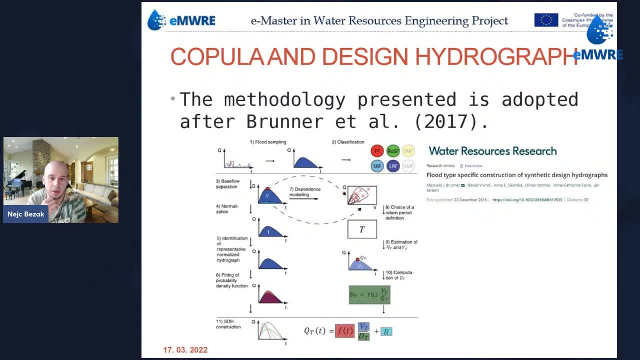 on web and find more details about how Coppola functions can be used in hydrology. I will now explain or present briefly another example, how this multivariate frequency analysis can be, let's say, a bit extended or upgraded. so if we do not want to basically use only the peak discharge information, but we 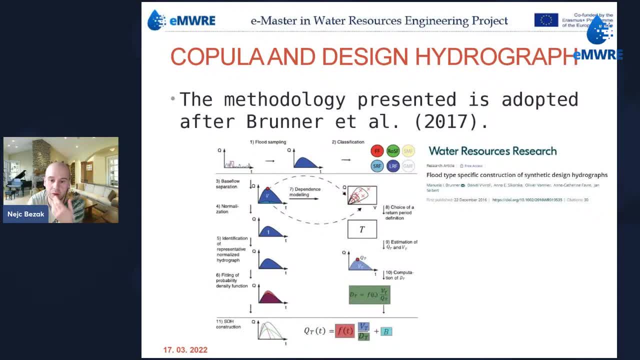 need the entire synthetic design hydrograph for our, let's say, hydraulic hydrological study, then perhaps this approach that was developed or suggested by Brunner in 2017 in the water resources research is something that you could use. so it's actually relevant, is simple. so these are the steps. so there are actually 10 steps that do. 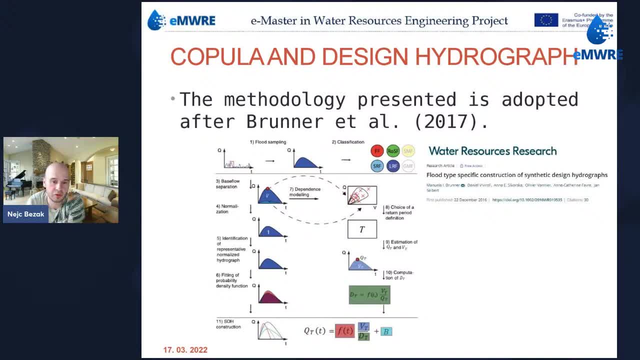 define this approach or this methodology. so the first one is this: the flood sampling. so here again, as I mentioned, either annual maximum or the picks over threshold methods can be used. then the second step is basically the classification of events. for example, if you have flash floods, if you, if you have 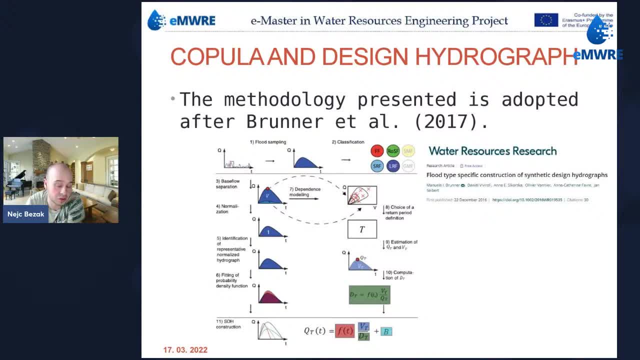 rain or snow floods, floods- if you have glacial floods or some some other definition, you can separate events into different classes. then you should separate the baseball, normalize the data in the defecate or like, say, our most representative hydrograph, you should fit the probability density function and 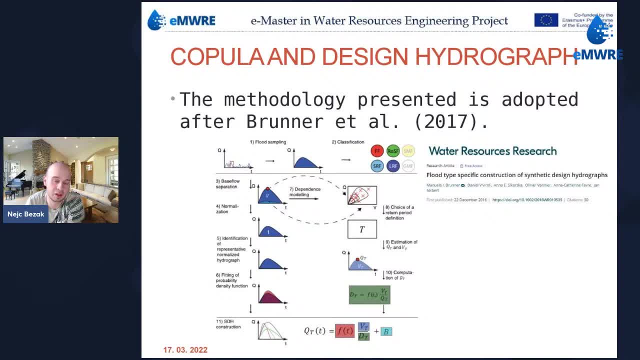 then here in the, in the step number seven, basically it comes the dependence model, so modeling the dependence between the pick if charges in the hydrograph volumes, and this is the step where Coppola functions can come into play. so it's basically the same thing as I. 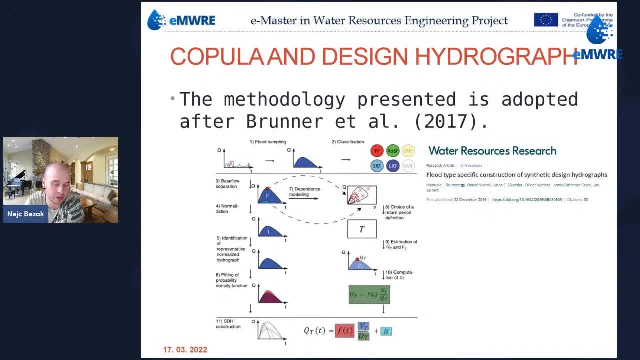 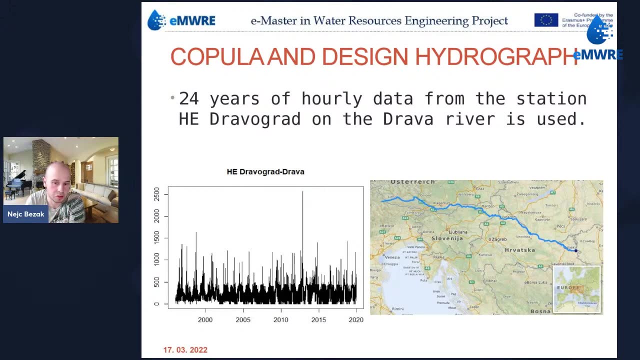 explained previously in my previous slides. I will explain another like example of using or applying this methodology to one of the Slovenian cases. so if you're not aware, so Slovenia is like relatively small country like that has around 20 000 square kilometers, located between Italy. 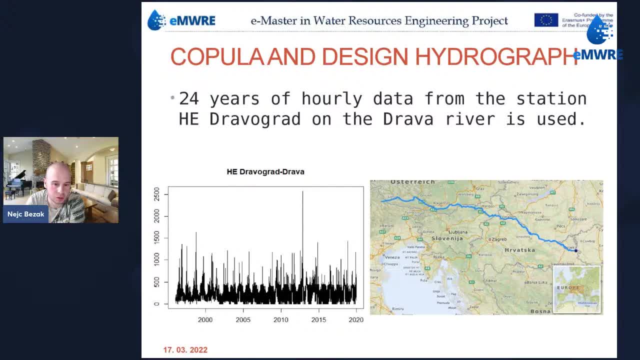 Austria, Hungary, Croatia. so in this case study, I used, like the discharge data, the hourly discharge data from the drama River, so Drava River is. so this is this blue line that you can see here on the on the screen- is quite big River that has its origin in Italy, then it flows to Austria, uh, and it also has some kind of 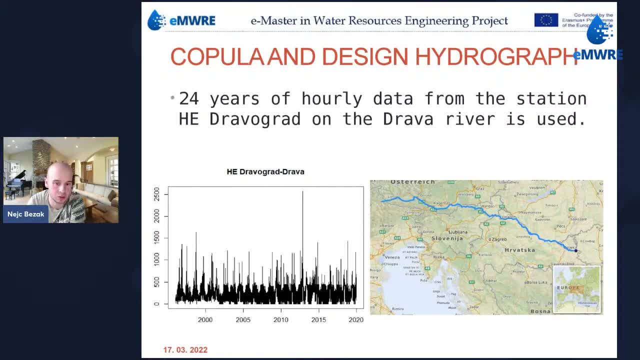 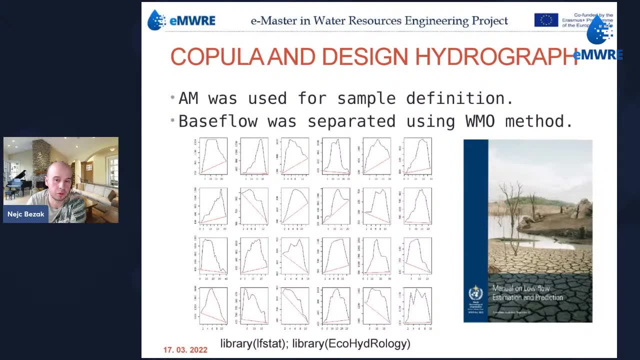 it also then comes to Slovenia. so this is the discharge data that I used from the Java River uh. so I did use the annual maximum method for for sample definition. I did separate the base flow using this board pathological organization uh methodology. so I did use the. if you're using the, the air software I I use, like 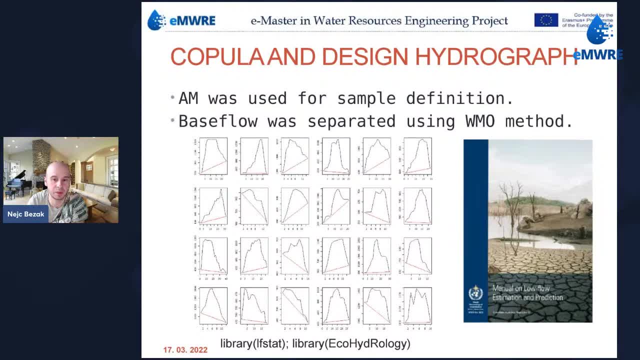 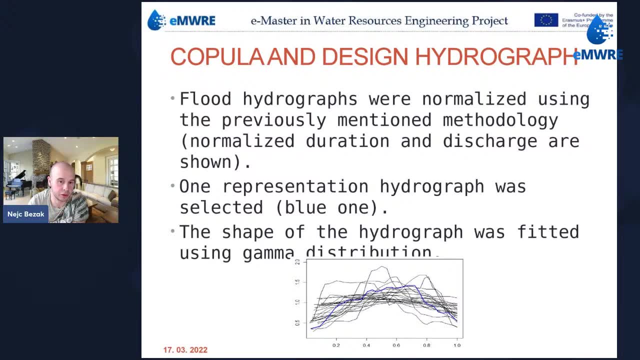 and eco hydrology packages to separate the base mode. uh, then I did the normalization of the data. I did select one representative hydrograph, so this is the one that is shown here on the on the graph. on the figure with blue line, I did describe or did, let's say, model the shape of the hydrograph using gamma. 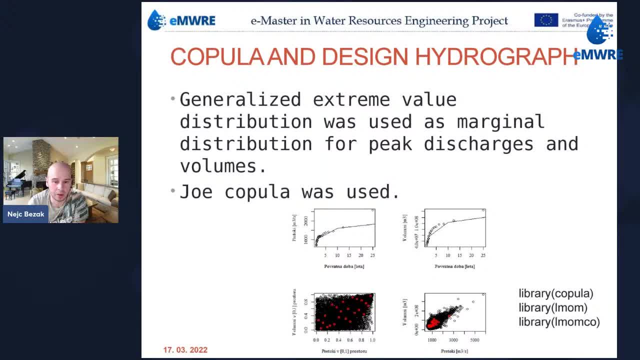 distribution. to make it a bit smoother, I did fit univariate or marginal distribution functions to both to the uh, to the peak discharges and go to the hydrograph volumes and I use Joe Coppola for modeling the dependence uh. I used packages, so air packages, Coppola, elmom and elmonco for for these steps. 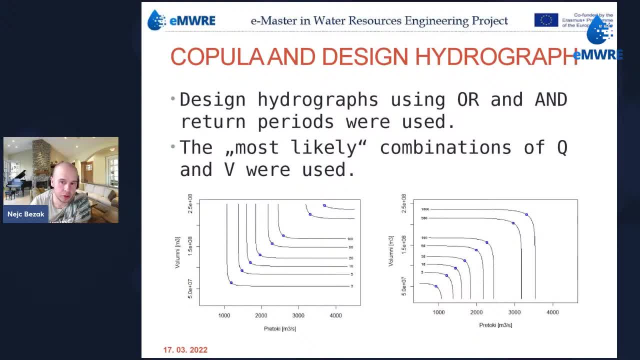 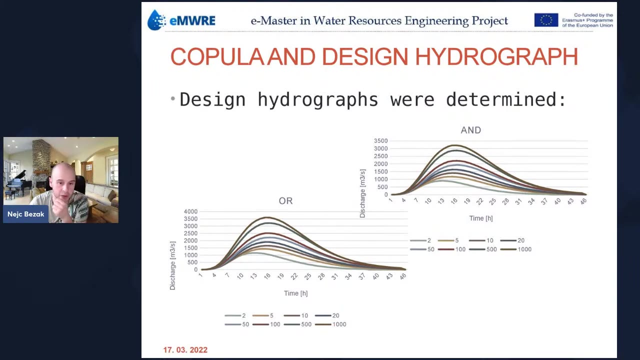 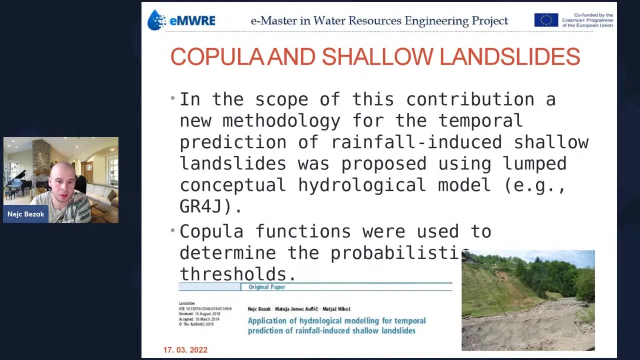 uh. then I derived or calculated the two return periods that I mentioned previously. so the air and owned and and I did select, like the most likely combination of of discharge and volume, uh for the for the definition of the design hydrograph. so these are basically the design hydrographs for two different cases, for different values of their therapy. um so, 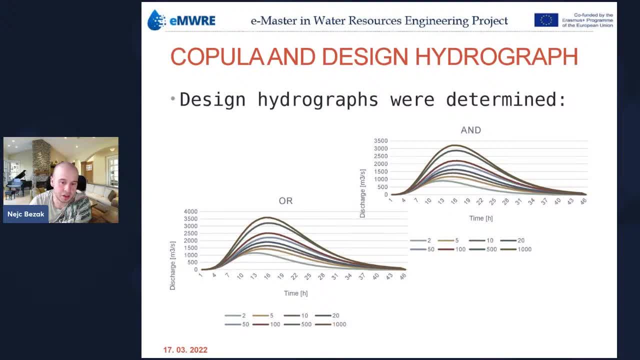 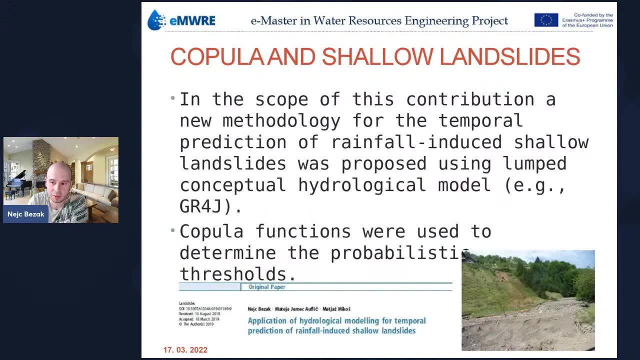 um, you can see that there is some difference and that, basically, the, the hydrographs for the all case are always higher. as for the end case, which is meaningful, and this like comes or can be uh understood from the definition of this return period. uh, I think that we are um. since we are, uh, I'm probably a bit late, so I will just briefly. 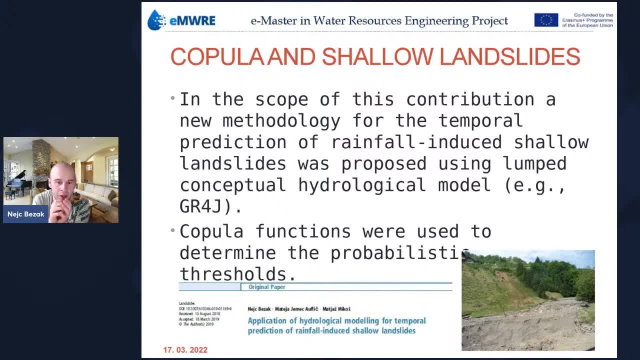 describe the second case study that I wanted to present. so, uh, as I mentioned that, as I mentioned, I'm also dealing with landslides, solar roving and stuff like that. so in this contribution- it was published in the landslide Journal- um, I wanted to use the hydrological modeling result for temporal prediction of 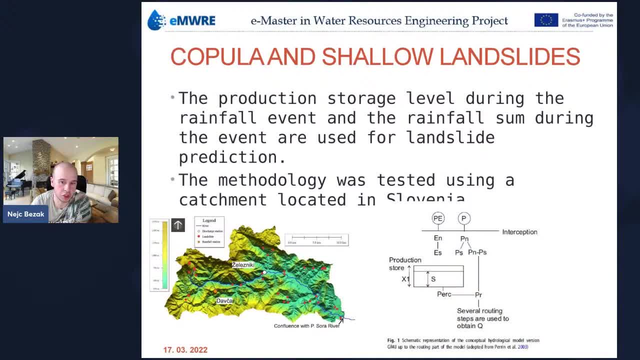 a rainfall induced shallow lenslights. so I actually used the French models of the GR4J for rainfall runoff modeling and then I used basically the volume of the water in this production store reservoir for prediction of the of the shallow main slides. why I use copula functions: 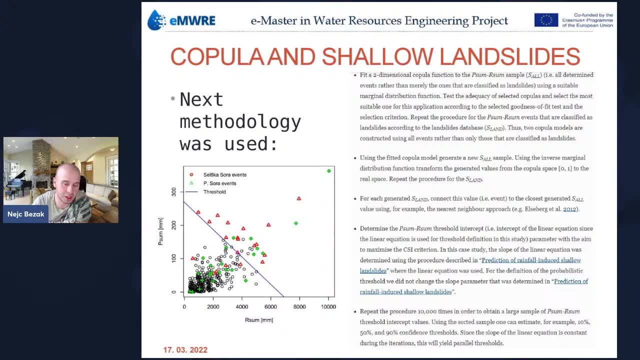 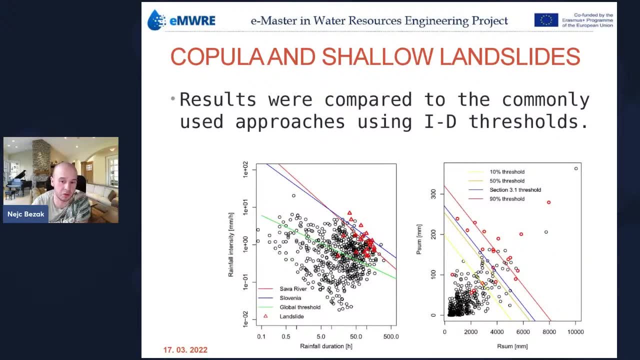 uh, so the the methodology, how it was done, is like this should be generated normally. foryora solution for practiced models would help to drawing described here, but I will not go that into details at the moment. So I did use Coppola function basically for the definition or for the development of the probabilistic thresholds. 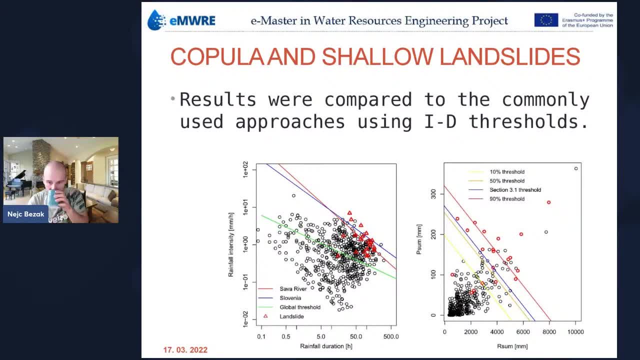 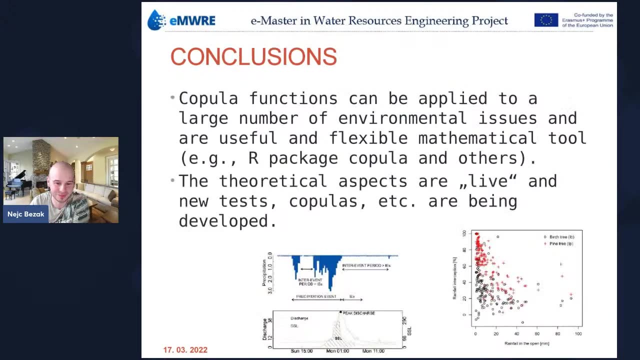 So these are the examples that are seen here on the slide. So I did compare these definitions with the classical definition of the empirical rainfall threshold. Sorry for that. Okay, so I have come to conclusions. So Coppola functions can be applied to a large number. 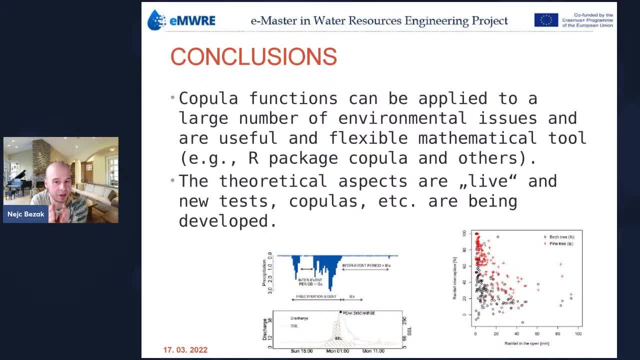 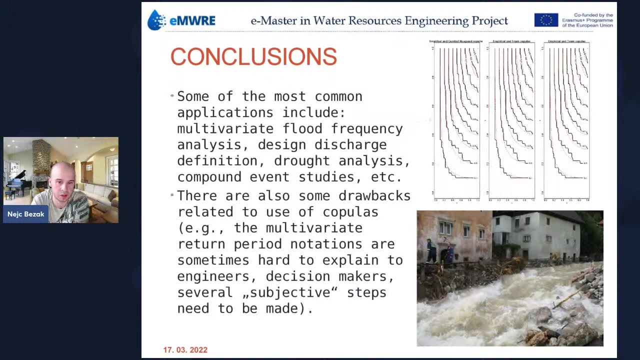 of environmental issues and problems and are flexible mathematical functions. To summarize what we just discussed, we can say that, debido to the fact that we have already discussed the phrase when we say that we have already covered the main issues, the behavioral issues we have already covered. the physical issues we have already. discussed with the mathematical tool. Even if you're not that skilled in math, there are plenty of packages already developed. So for example, in R, this is package copula. there are packages in MATLAB and other in other software, As I said. so theoretical aspects are live, So the Coppola functions are still under development. 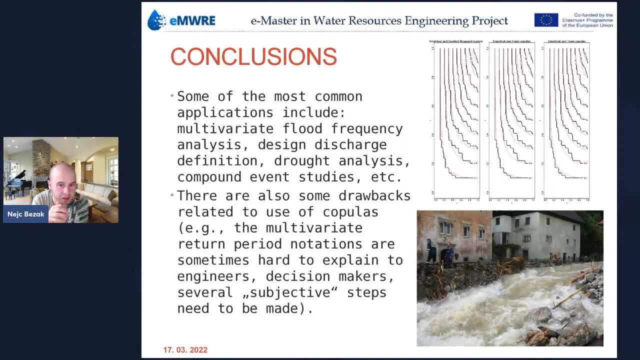 New tests, Coppolas, are being developed by the mathematicians. These functions are not only used for the multivariate flood frequency analysis but, as I mentioned, they are often used for drought analysis, for compound event studies, etc. We must be aware that there are some drawbacks related to the use of COPPAs in hydrology. 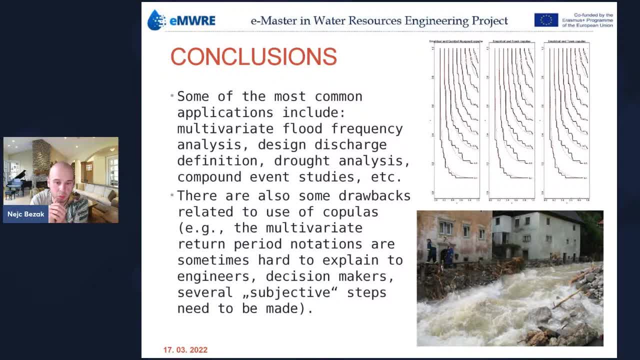 So there are some subjective steps that need to be made, such as multivariate return period notations, multivariate return period definition needs to be selected, marginal distribution functions need to be selected, base flow method needs to be selected, etc. And some of the steps or some of the results are perhaps sometimes tricky to explain to decision makers, engineers, different stakeholders. 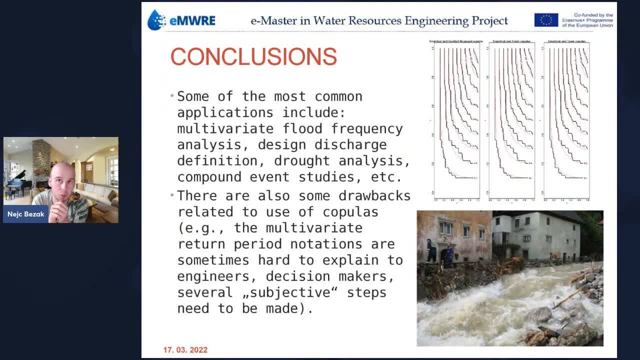 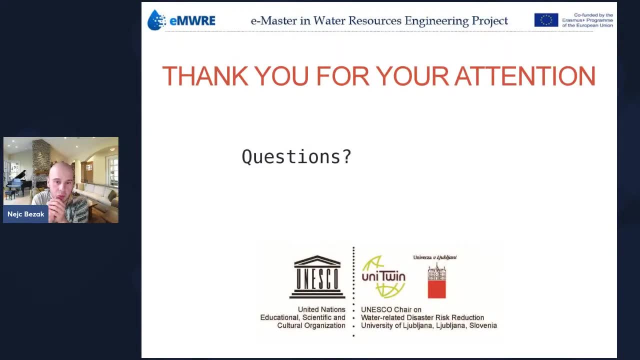 So especially the notation of the multivariate return period is perhaps the most tricky part. that should be really well presented to these people. So that's more or less all from my side. So if there will be any questions I'm happy to answer them. 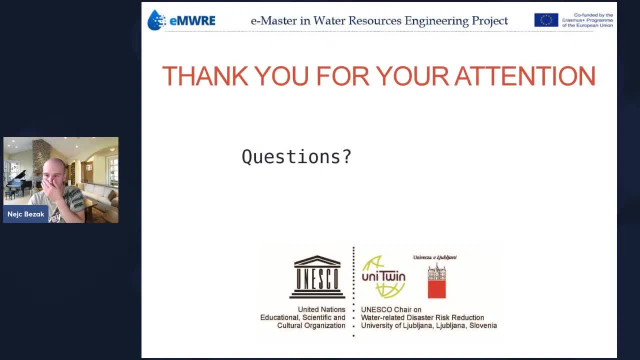 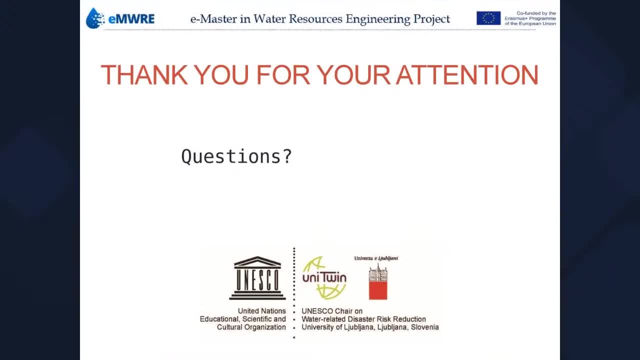 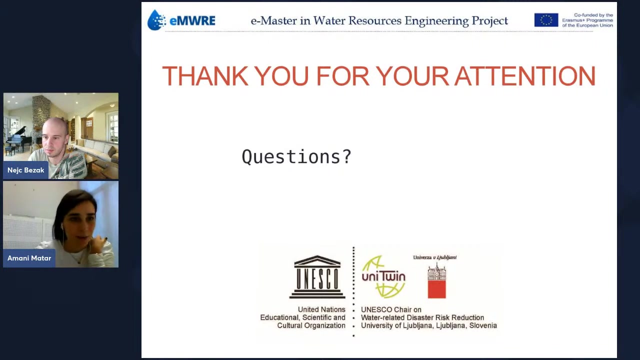 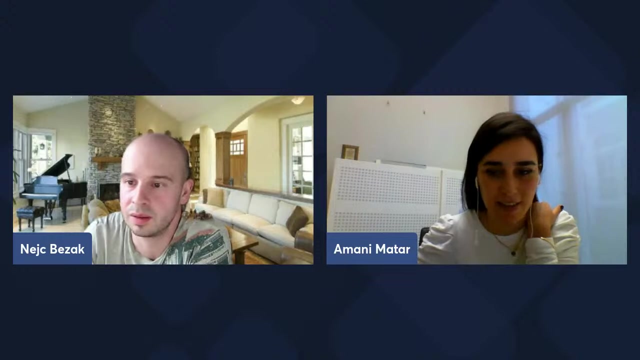 Thank you very much, Dr Roenick, for this presentation And I hope you enjoyed it. I hope everyone enjoyed it And please ask your questions in the chat box if you have any questions. So we have a question. There is one. I can see it. So how do you select the COPPA function? 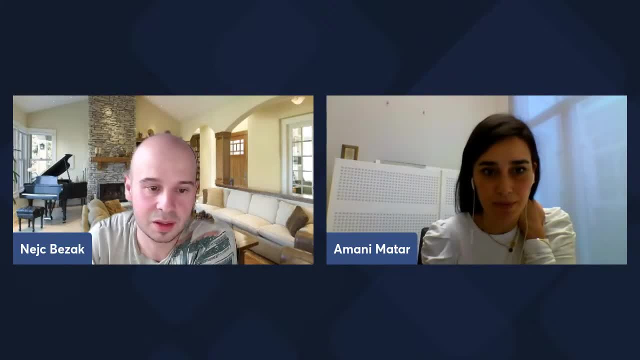 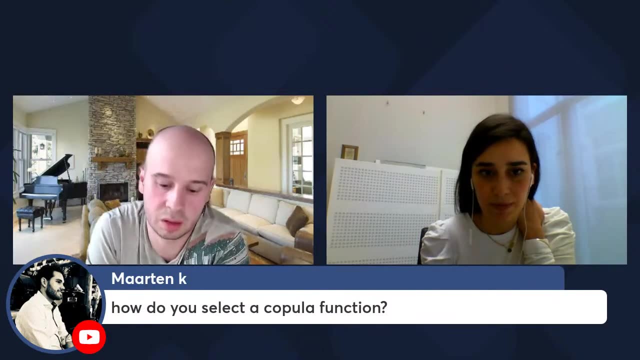 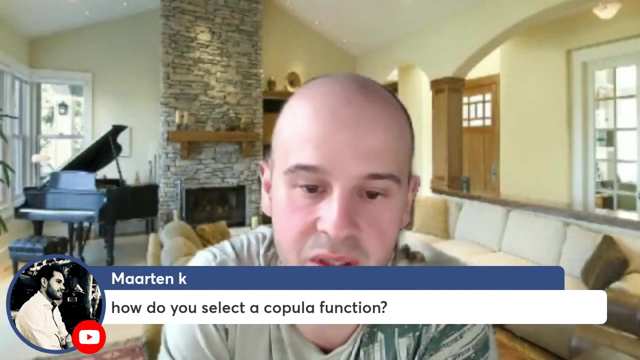 Yes, So there are. as I said, there are different statistical tests with which you can learn, Like, let's say, reject or not reject the COPPA function, And there are different, like graphical tests that can be used to double check if the selected COPPA does fit to the data. well, 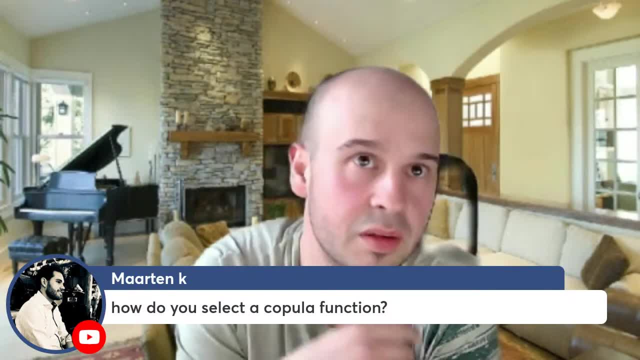 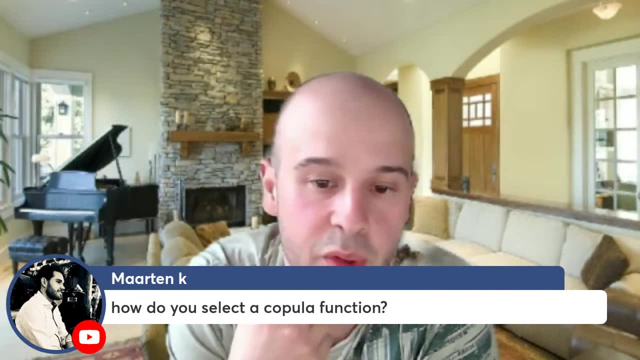 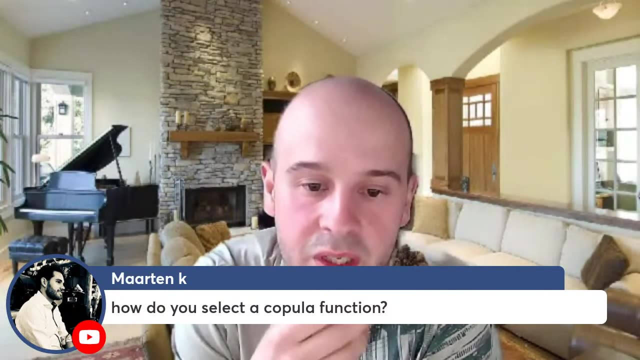 So there are the tests. some of them- like they are, like they have the names, like for Mises test is one of the frequently used- are also implemented in the previously mentioned error packages. So, for example, the COPPA package does basically also include some of the tests. 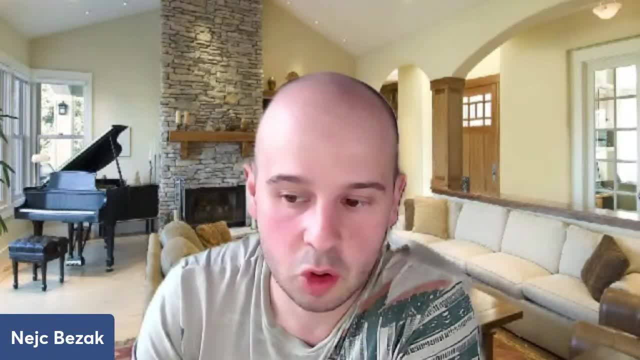 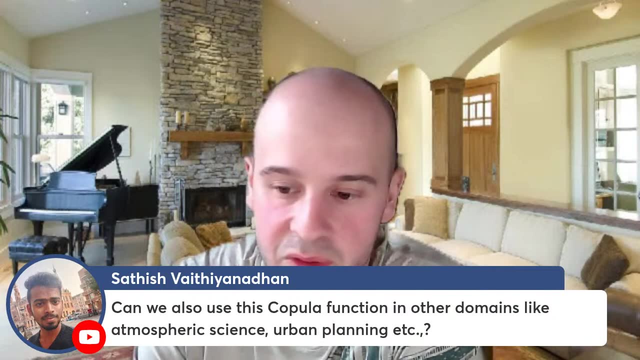 So the next question, I think, is: can we use these COPPA functions in other domains? Yeah, sure, So as I showed in one of the slides, one of the early slides, COPPA functions are not only used in environmental engineering, which I think it only came fifth on the list. 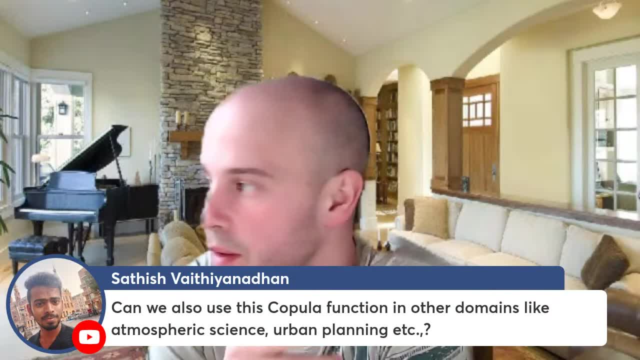 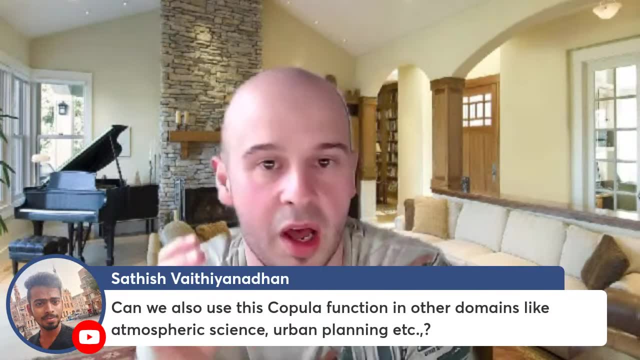 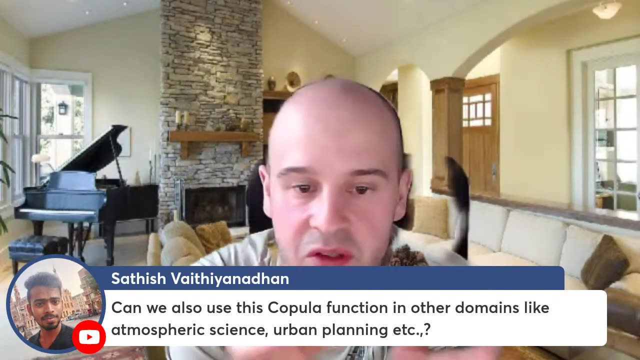 But there are other fields like computer science, economics, where COPPA functions are also used. So basically, if you have like two variables, two things that you would like to combine, and there is some dependence between these two parameters, variables. 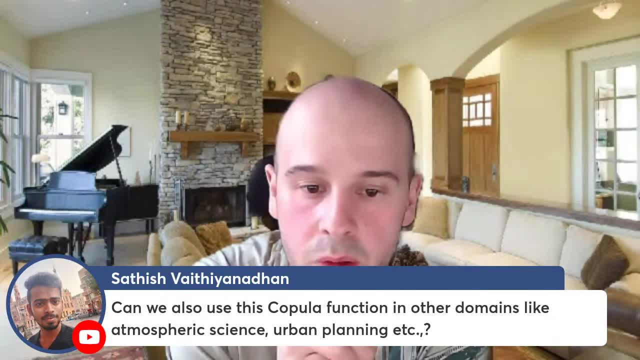 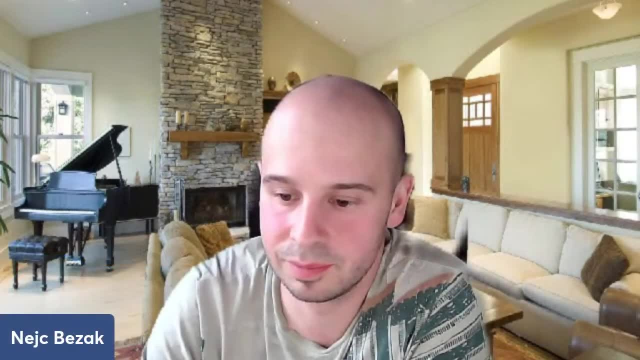 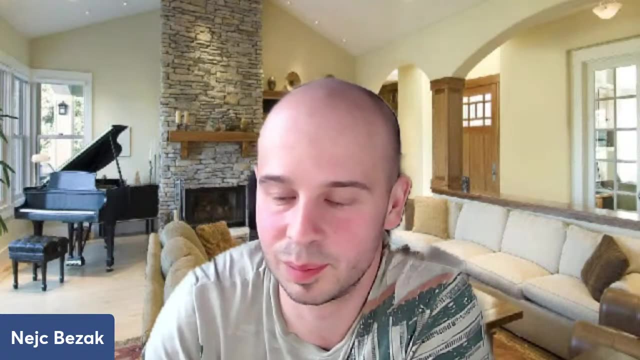 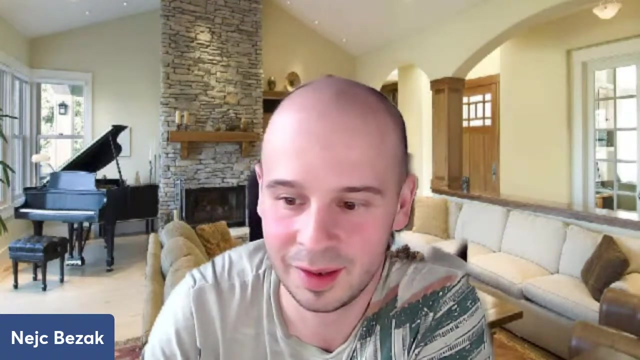 then the COPPA functions are used. So these are probably good tools to test and use COPPA functions for modeling. So I think I hope I answered the question. If there is anything else or any other question, just let me know. Thanks, 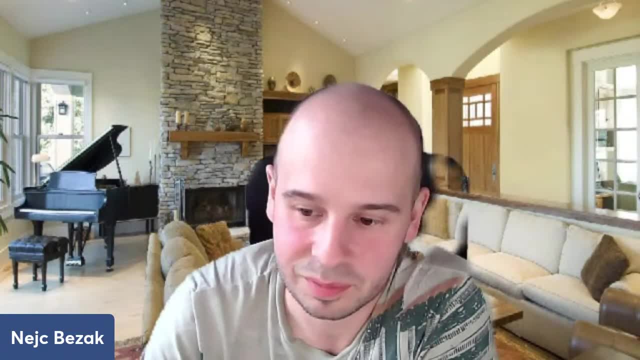 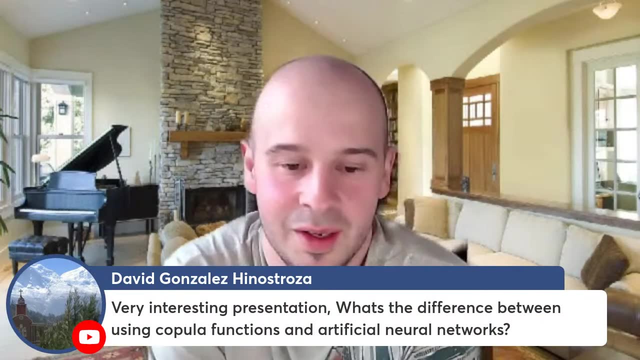 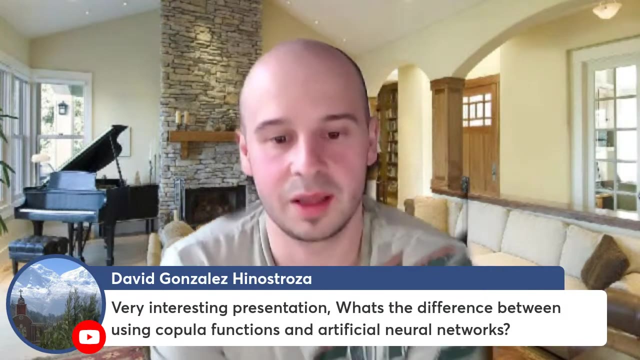 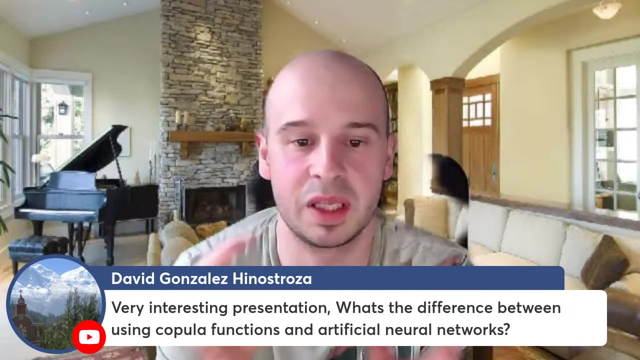 Okay, so yeah. the next question is: what's the difference between the using COPPA functions and artificial neural networks? So I'm not that big expert in artificial neural networks, but COPPA functions are basically the mathematical expressions that are very explicit. 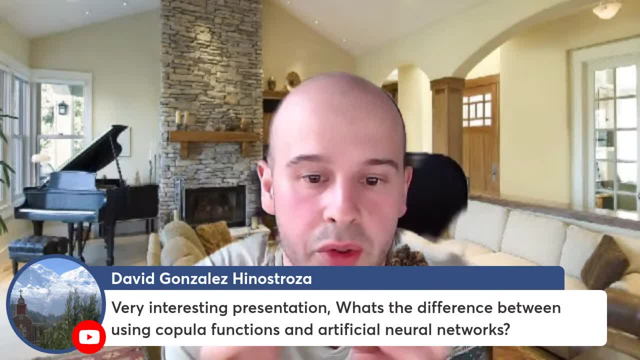 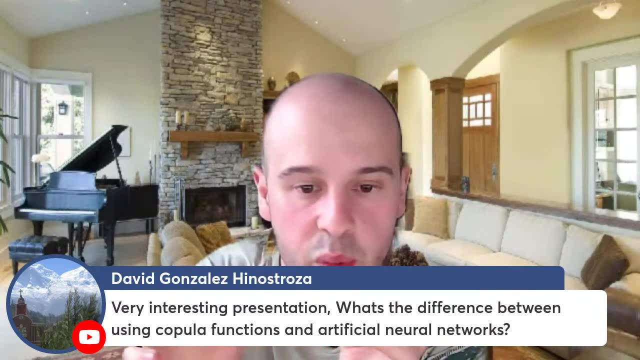 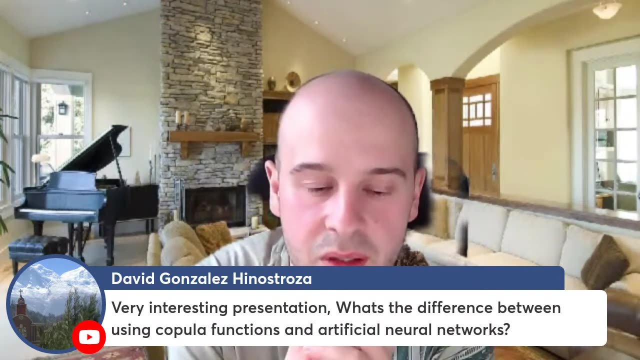 So you basically know. you basically know what you're using, while the artificial neural networks do develop like some connection between the data sets. So there is some. there is some difference in the between both two tools. So the COPPA functions are actually very, let's say, core statistical tool that can be applied to almost any type of the data. 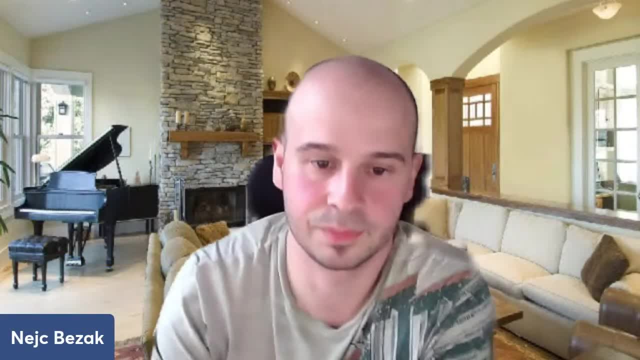 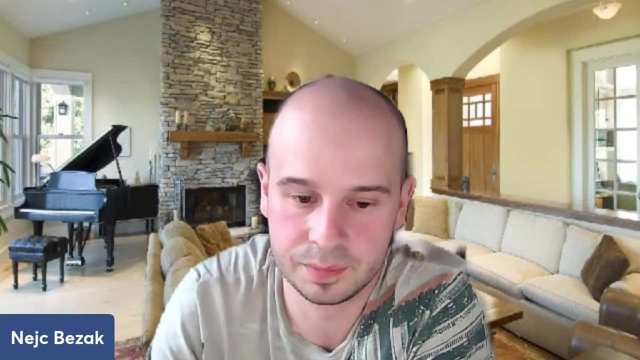 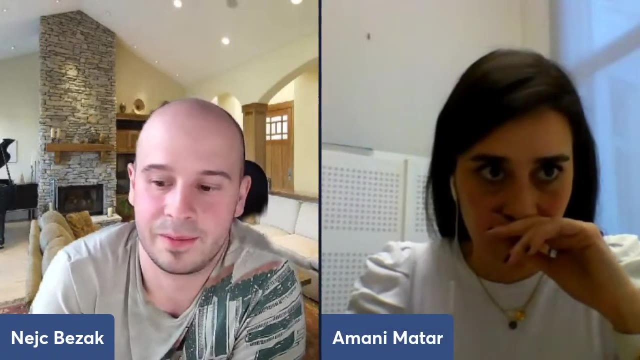 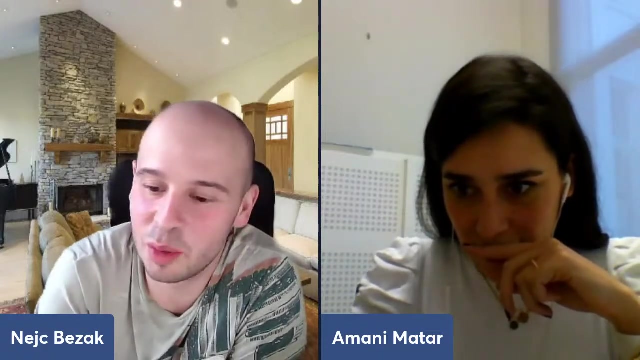 So that's Yeah. so perhaps another question- It is more like technical one, So will this video stay up on YouTube? I think it will right. Yes, it is. So you know like yeah, so I guess pass it on to Angelica. 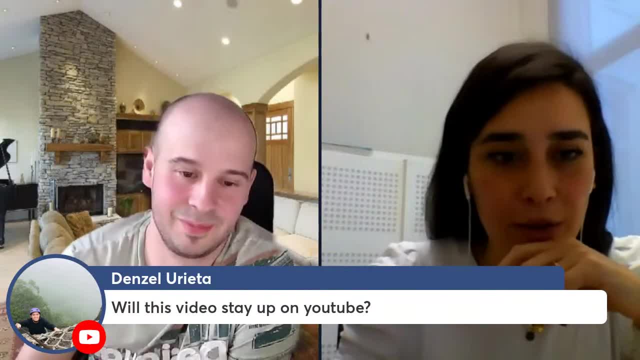 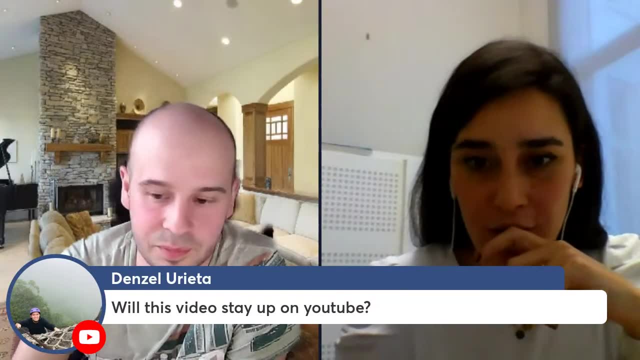 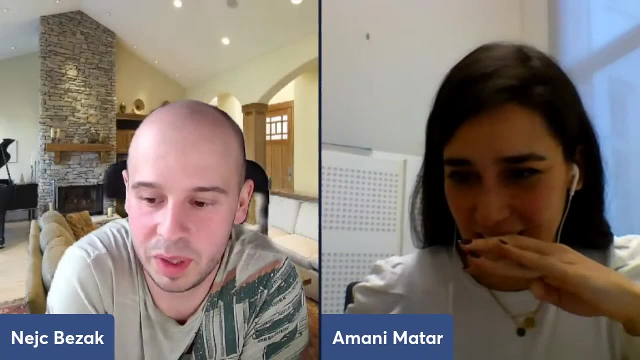 Yeah, I just said this one. Yes, this video will be on YouTube and you can also see and see all the project updates on the project website. It's also posted on the chat. Okay, we have another like For you. Yeah, question: how big should the data set be? 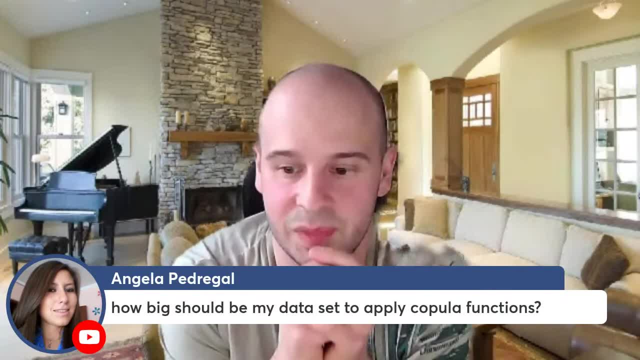 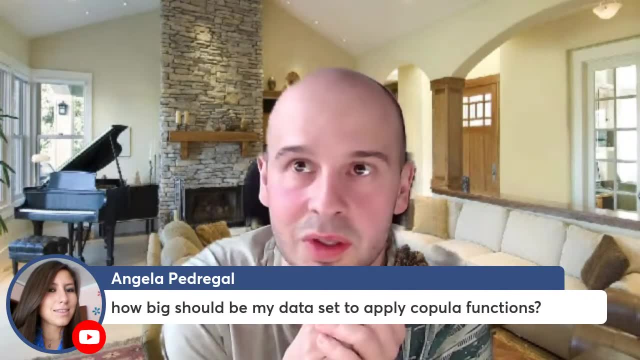 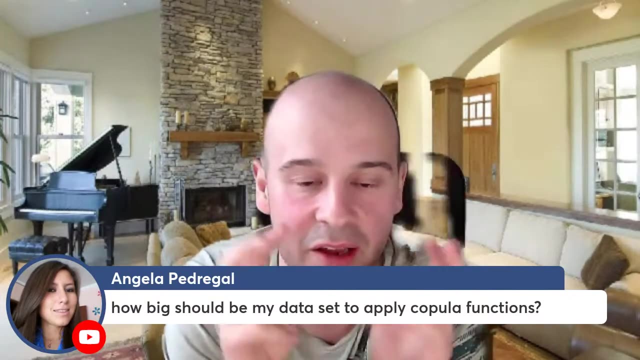 to apply the Coppola function. Yeah, so basically, like there is no like formal minimum, but I suppose I would say you need to have at least at least like minimum 20,, 25 points, or let's say events, to adequately fit Coppola function. 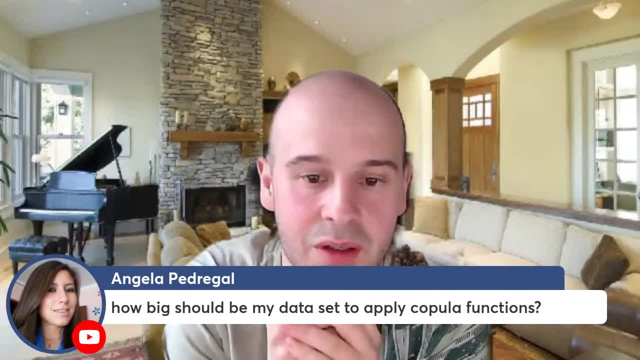 So it's similar as in the case of the univariate flat frequency analysis, where also you need to have- I don't know- at least 10 or 15 years of data to do it. If you have only 15 years of data, 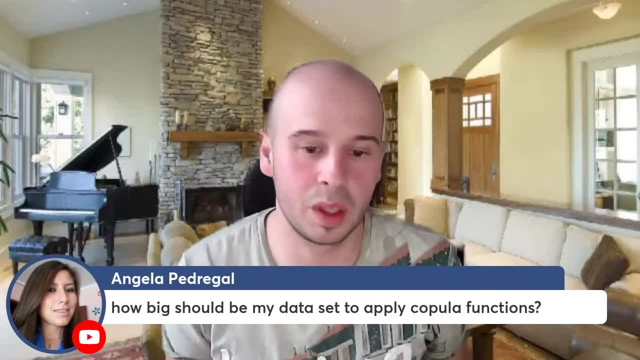 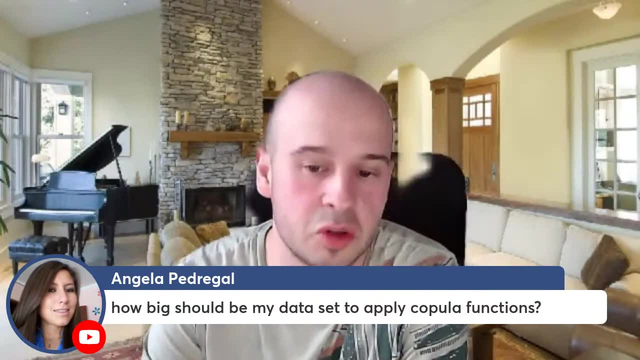 if you have only two or three events, you can basically extend the sample using I don't know extend of using picks over. instead of using annual maximum method, you can use the picks over threshold method, for example, And in this case you can like make the sample. 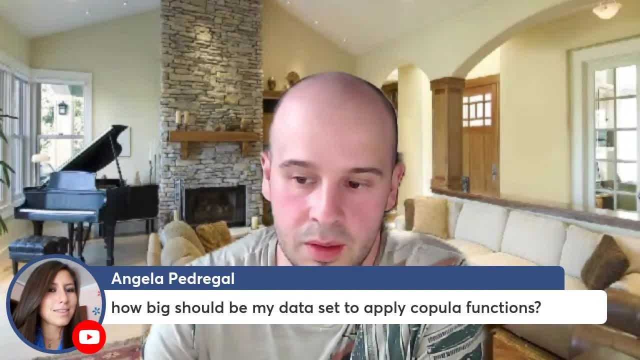 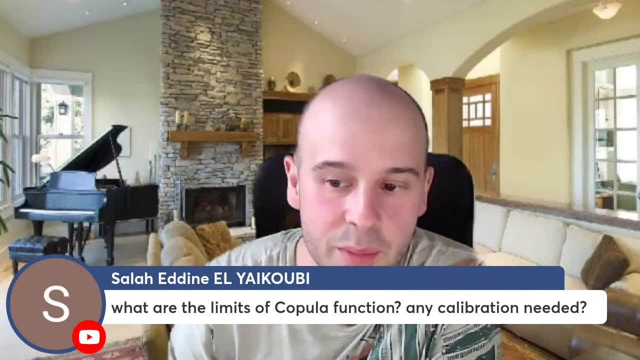 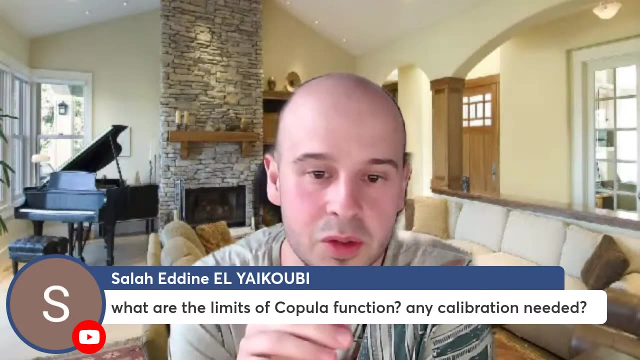 that you have bigger. So the next question is: what are the limits of Coppola functions? calibration needed? Yeah, so the Coppola function parameters. so in the b-variant case. so this is the most simple one, where you have pick, discharge and the loading. 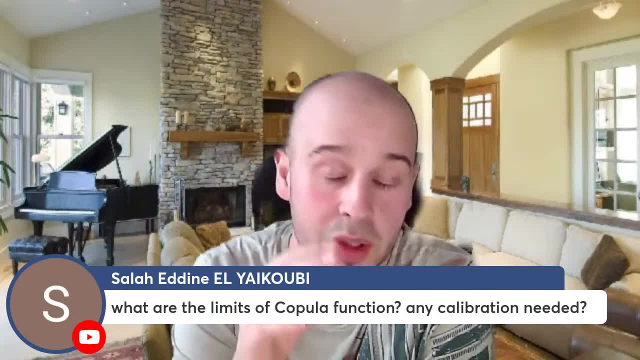 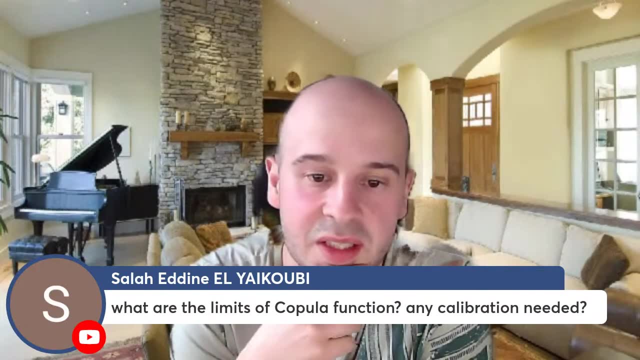 you need to estimate the Coppola parameters. So the Coppola- so at least the Coppola that I shown on the screen- only have one parameter. So there are similar. as in case of the univariate case, there are different methods available how to estimate this parameter to get like the best fit. 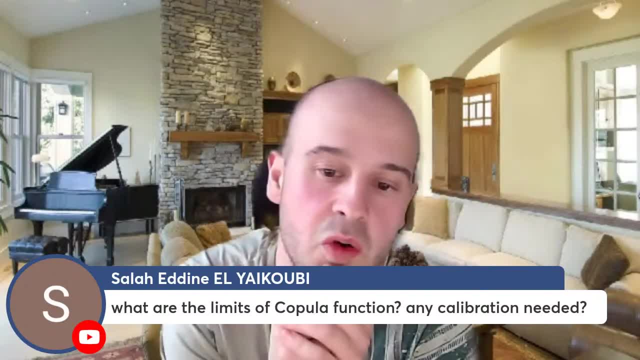 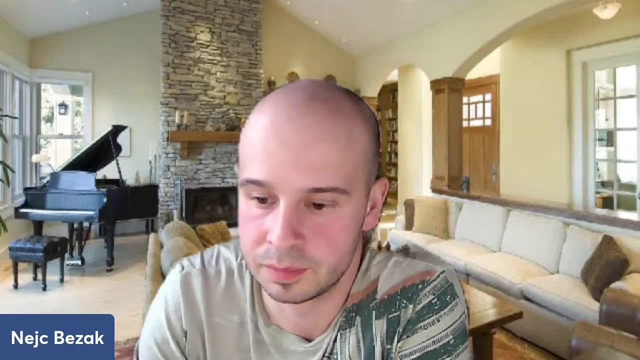 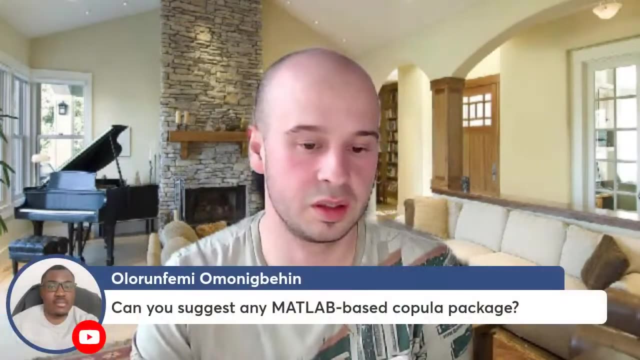 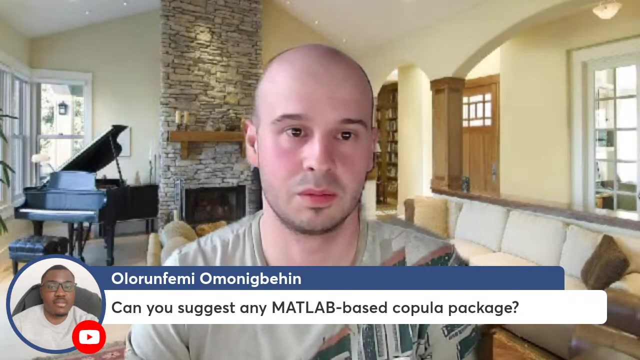 of the Coppola function to the data you have. So this is the calibration, the Coppola function, of course. yeah, So- There's one more. Yeah, there is some MATLAB-based Coppola package. I can Google it quickly. I'm not sure, since I do not use. 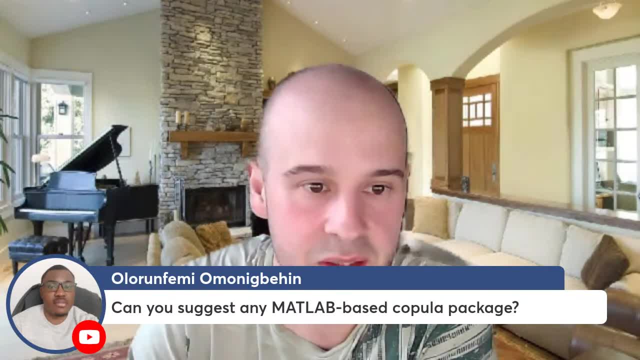 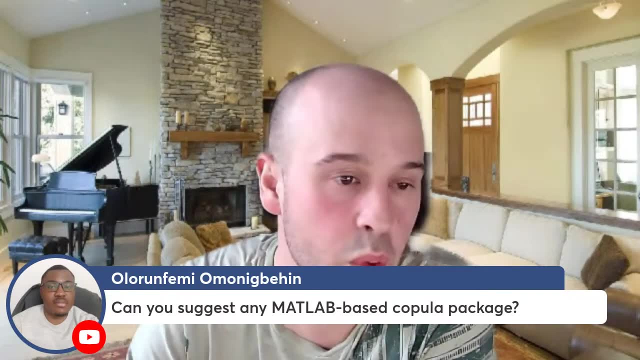 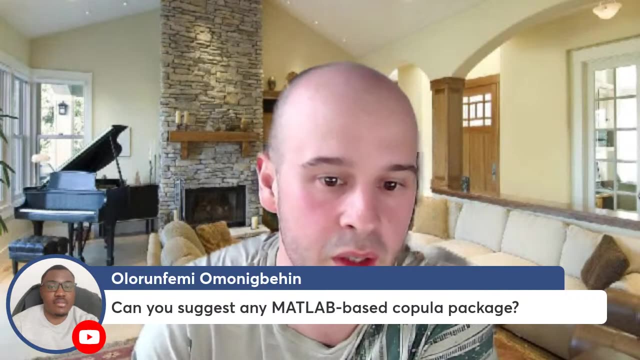 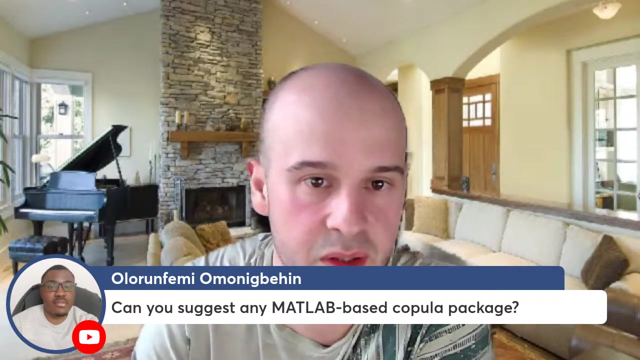 MATLAB, I think it's. if you search like Coppola fit, this should be one of the functions in MATLAB and then you should probably be able to to find which. what's the name of the package, I suppose, But if you're interested, 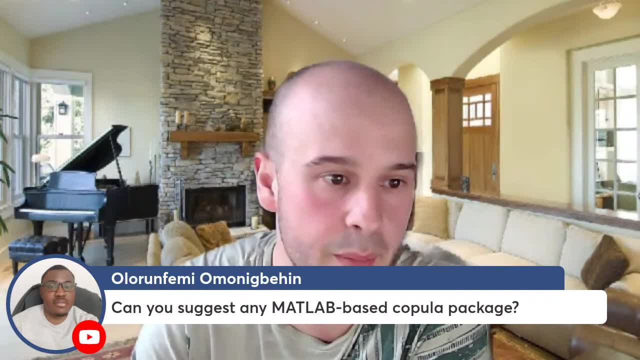 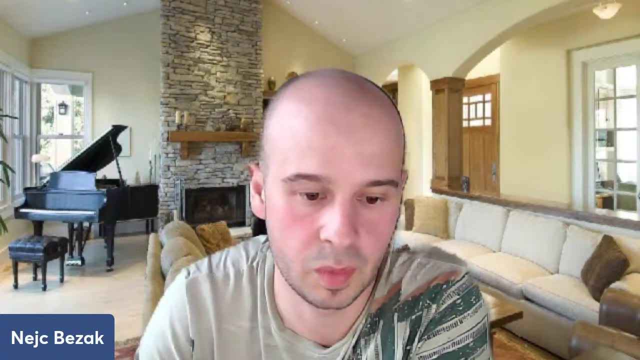 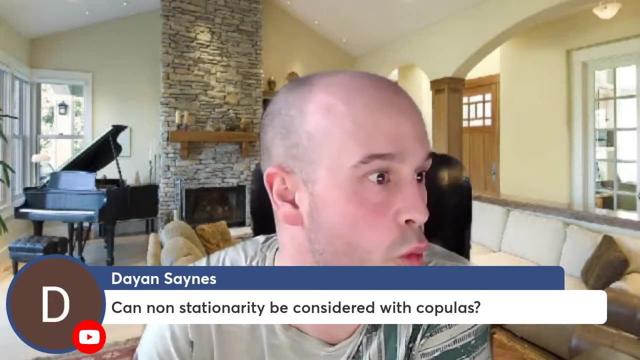 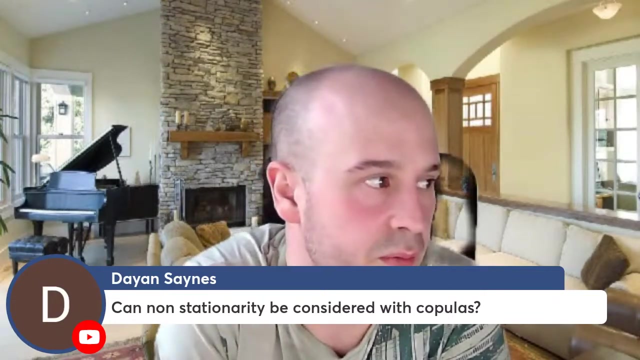 I think it should not be that difficult. if you Google like MATLAB and Coppola, there are plenty of search hits. And then that's another one. can non-stationary be considered with Coppolas? I think yes. to be honest, I have not yet like. 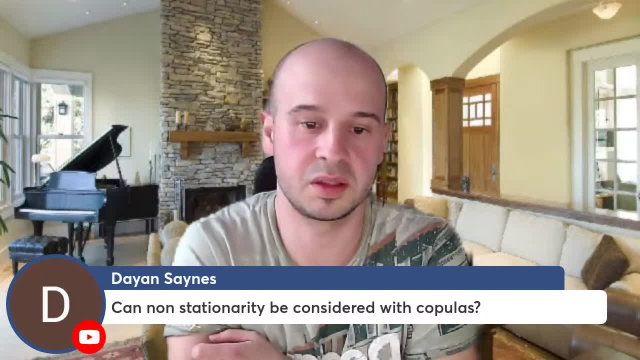 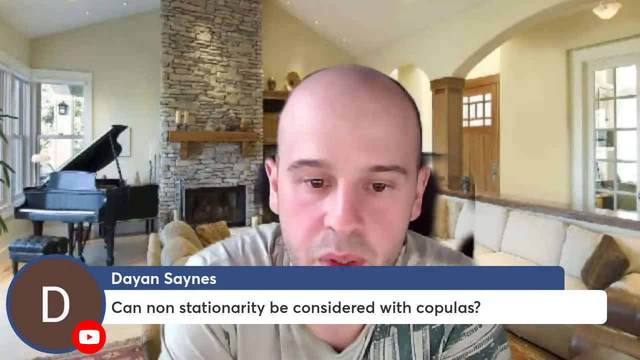 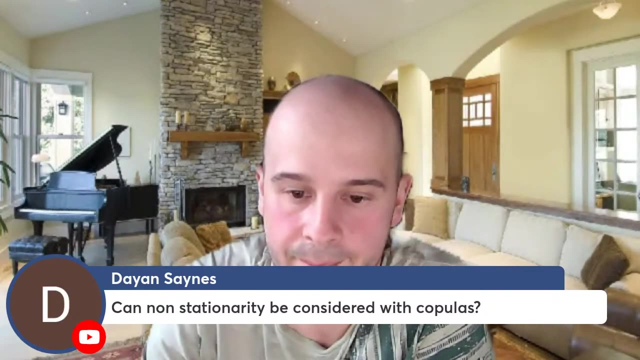 detected paper or study that would use like the non-stationarity methods in relation to Coppola functions, but I think this should be like something that could be done, of course. So the next question is: can you use Coppola function to determine the water quality? 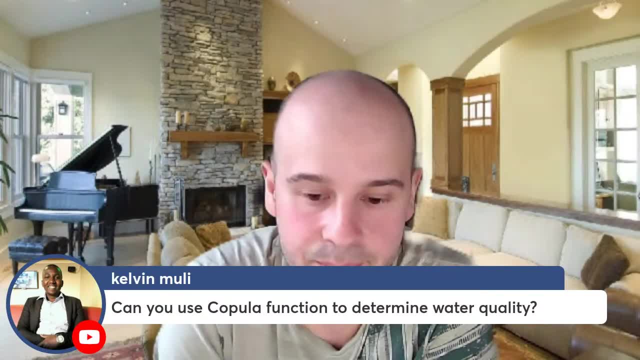 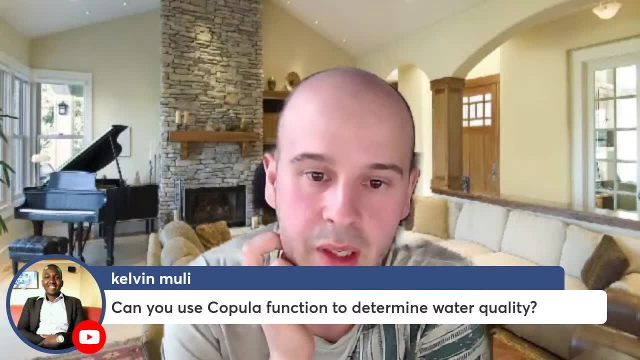 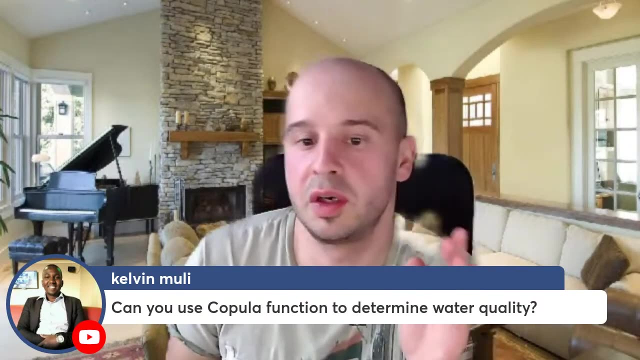 So if you have like the water quality data and you have different parameters of the water quality, then Coppola functions could be used like to model these dependents and perhaps make, for example, if you're measuring, two parameters for some period you can fit in. 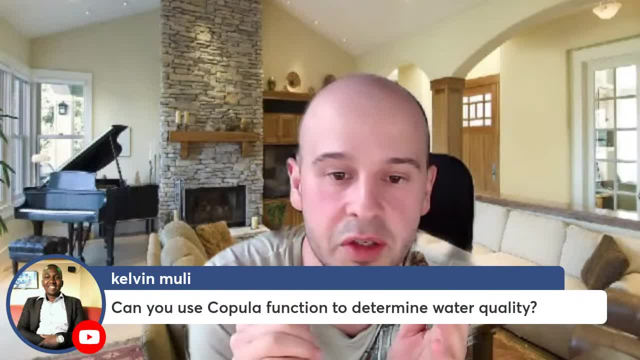 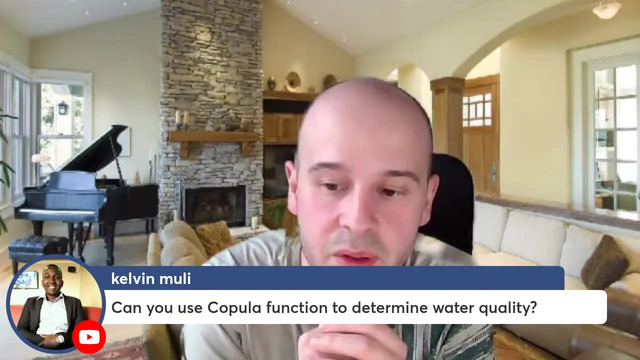 let's say, calibrate Coppola function and then you stop measuring the second parameter, then you could use such Coppola model to estimate, basically, the parameter that you're not measuring. can you more? we, based on the measurements of the parameter, the parameter it is still measuring. 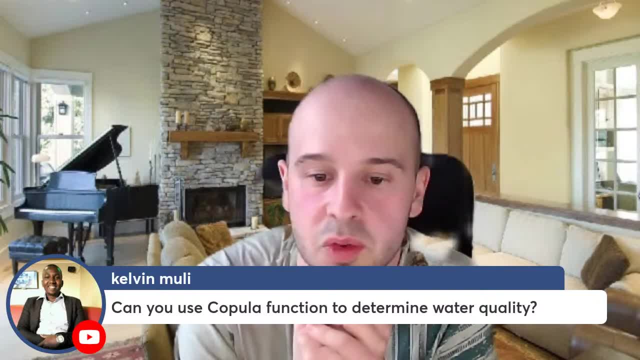 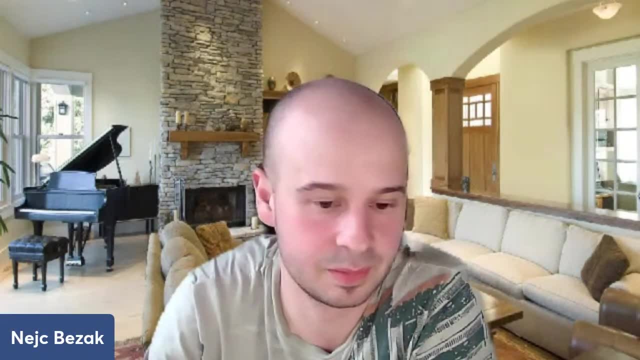 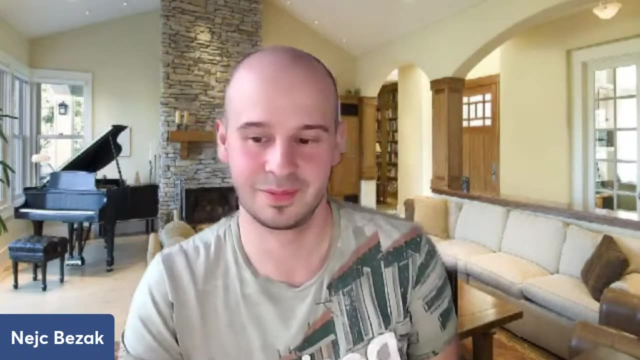 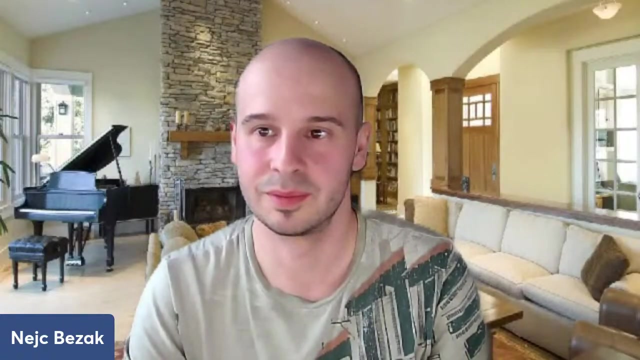 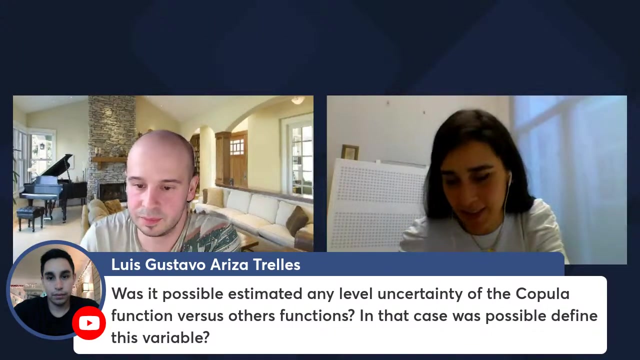 So this would be one example how Coppola functions could be used in relation to water quality, of course. Thank you very much, doctor, for this. I think more questions are coming in. There's another one. okay, I believe. now that's good. 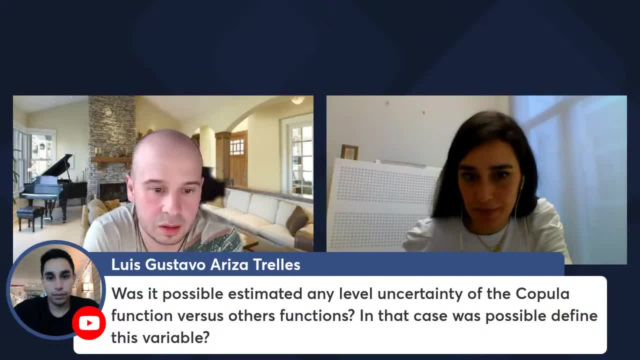 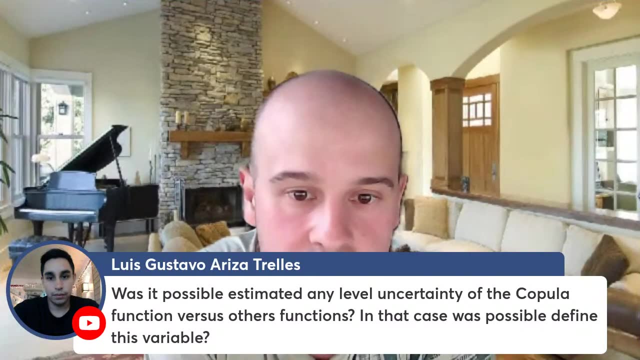 Yeah, sure. So if you would like, would want to make like a robust estimation, then estimation using Coppola function should be like associated with water quality, like some estimation of the uncertainty. for sure, this could be like done with like some probabilistic. 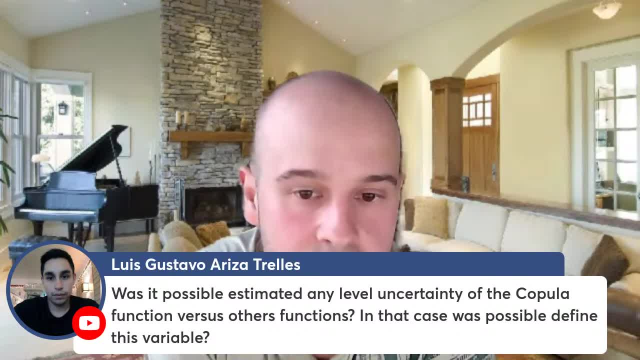 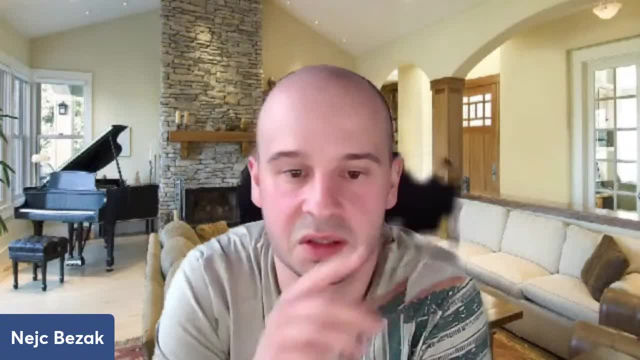 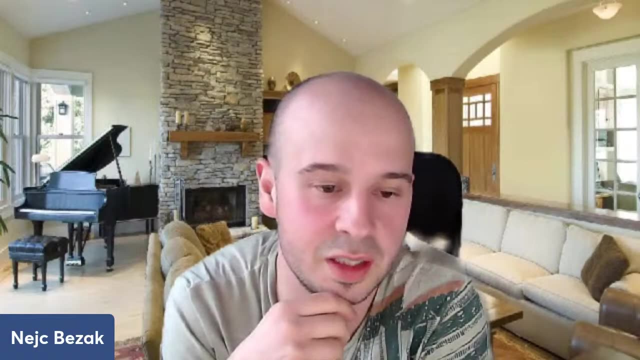 methods like uh, similarly as, as i showed in case of this shallow lens slides, just briefly. so this is like uh, this threshold. there were, if you can remember, like three thresholds were were shown: the 10, the 50 and the 90 thresholds. so this 10 and 90 thresholds are basically. 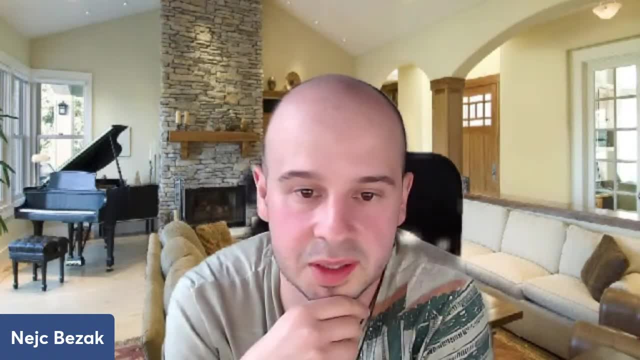 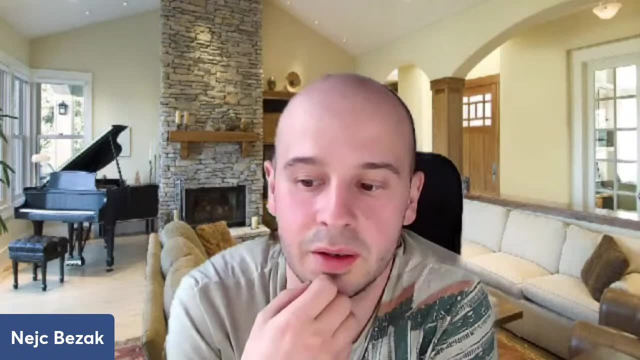 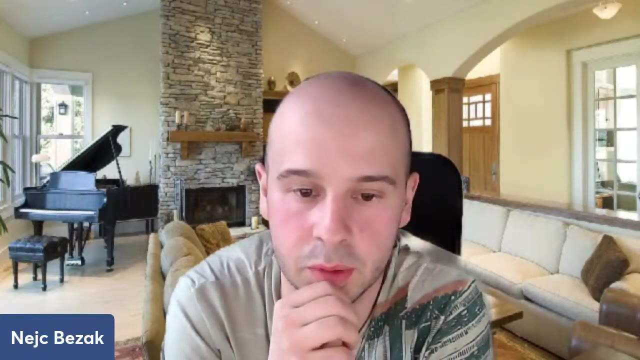 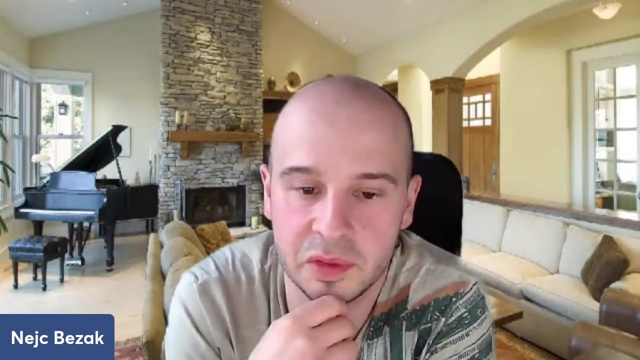 uh, let's say an indirect estimation of the uncertainty of the derived or the copula function result. so similar thing or steps can also be done in other applications, like multivariate frequency analysis or water quality, for example. for sure, yeah, and like, if you're asking, like comparison of the uncertainty of copulas with other like tools, 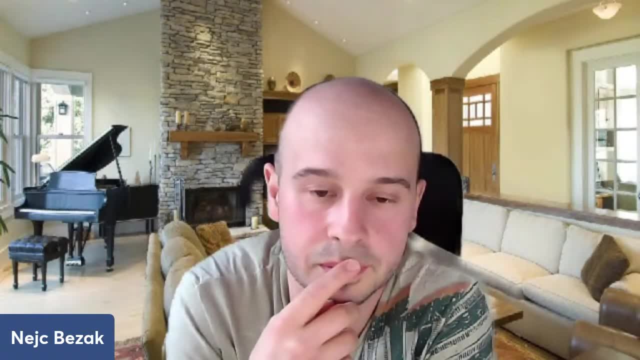 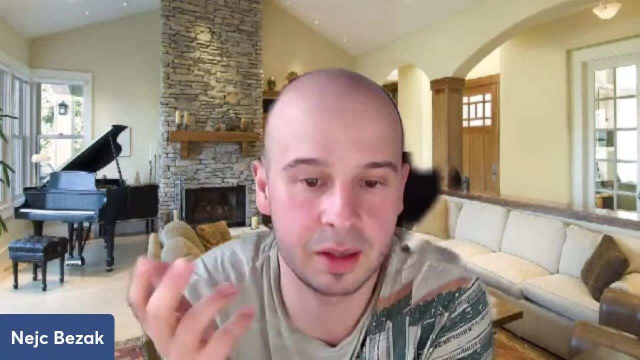 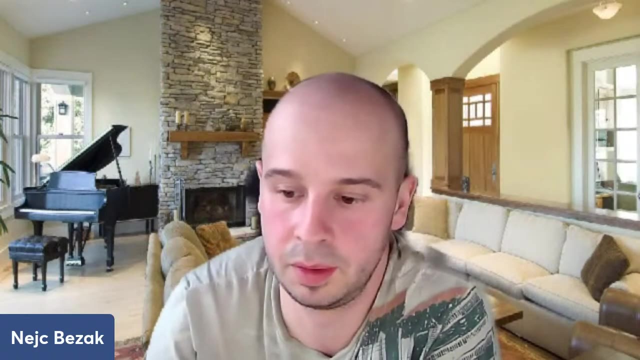 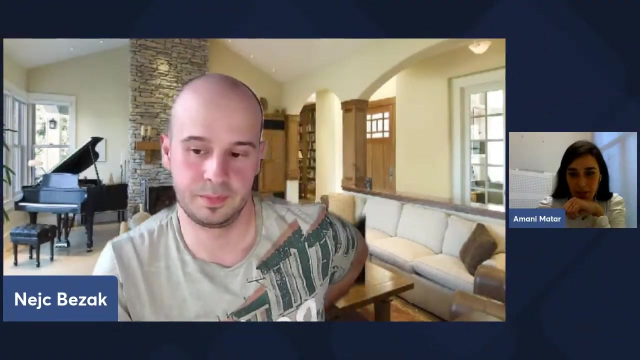 or methods, then it, of course, depends on the um. it depends on the characteristic of the data set that you have, so it can occur that any, perhaps some other method or or tool will better fit the data that you have and there will be smaller uncertainty. okay, thank you very much and thank you everyone for your questions and for interacting in this. 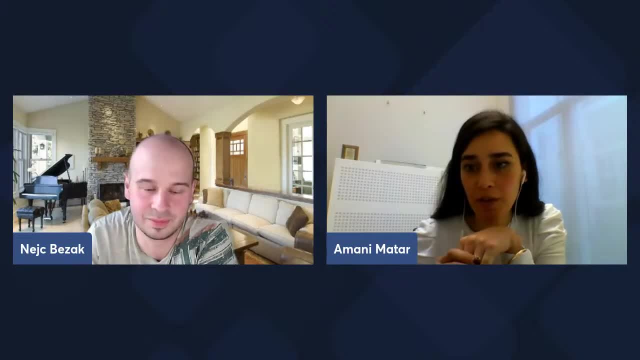 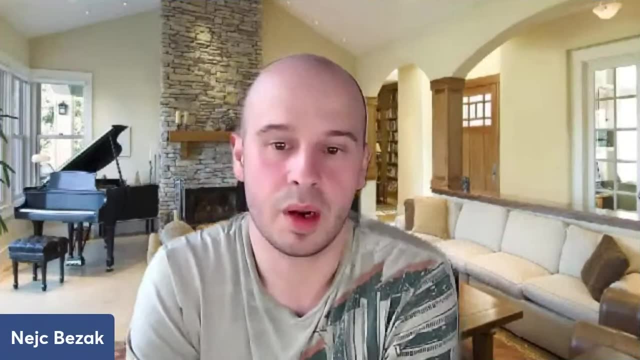 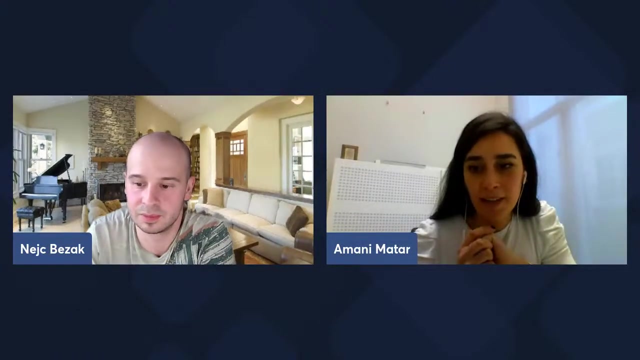 session. um, i would like to say: if you have more questions, you can send them and we can share them with the presenter and reply to your answers after that. um, i think it's time to end our q a, but thank you everyone for joining and it was really nice to see your presentation as well. 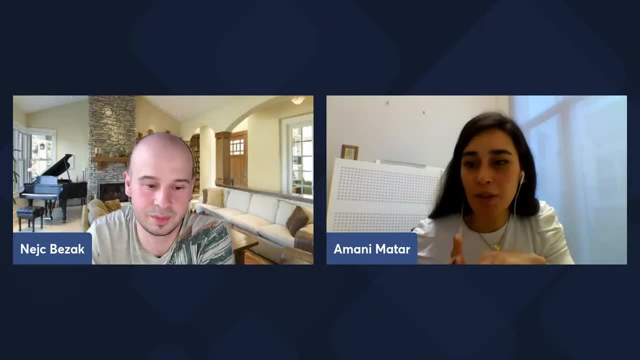 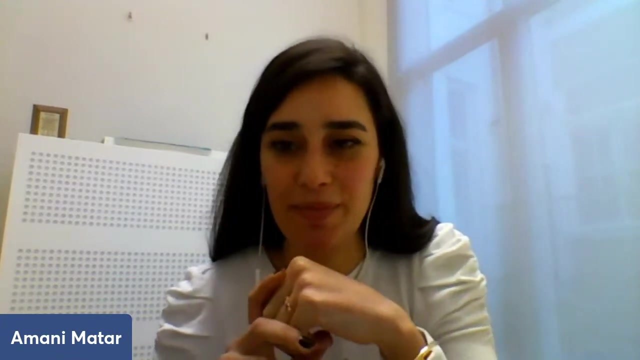 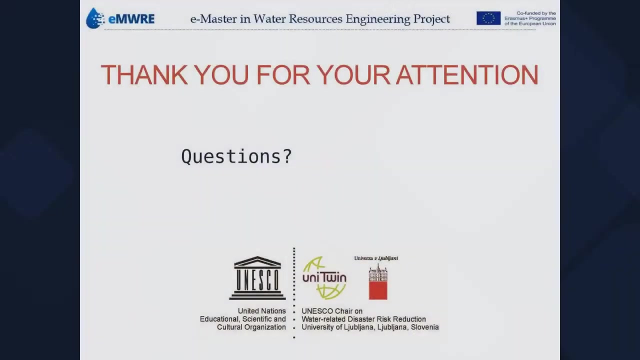 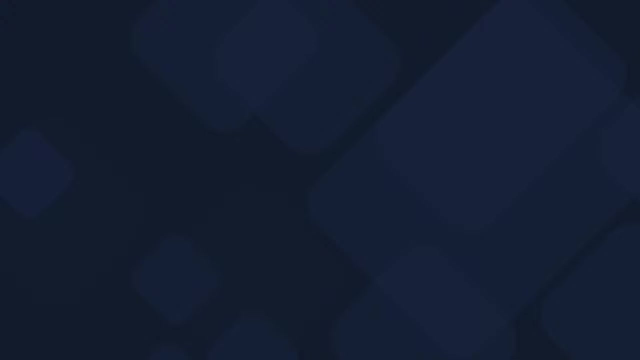 doctor very interesting and we're looking forward to see you in our next webinars as well. for this webinar series from the project. so thank you everyone and we hope to see you in the next webinars. thank you you.